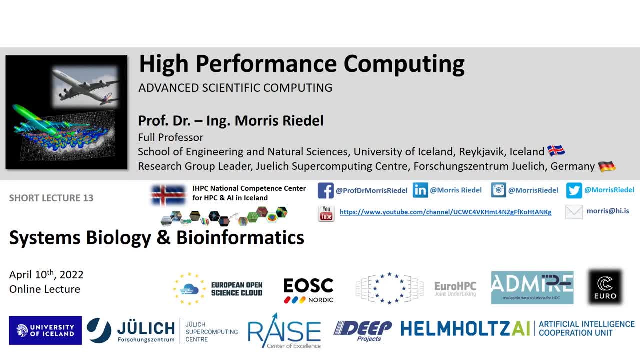 Welcome to High Performance Computing, Advanced Scientific Computing. Today we have our short lecture 13 about systems biology and bioinformatics and it's really continuing in the idea of our lecture series that we have now basically, in the first part of all the course, understood: MPI, OpenMP, the role of GPUs. 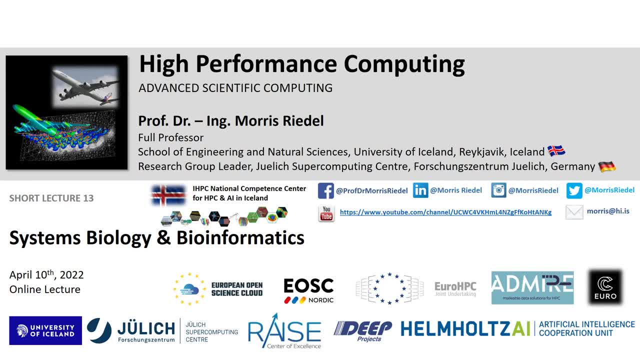 accelerators and CPUs. And now we want to understand more in the second part that we already started with essentially, with short lecture 11, with 12, basically on CFD, on health applications, really to understand where HPC makes a difference and which application. 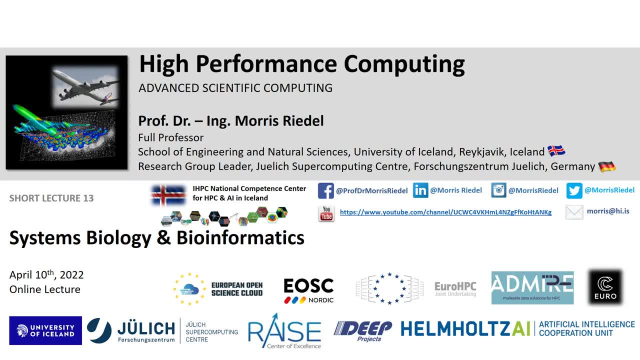 fields. These are, of course, more or less short lectures. So if you really want to be experts, for instance here in systems biology or bioinformatics, you really should study a complete course on these topics, And here at the University of Iceland. I would recommend. 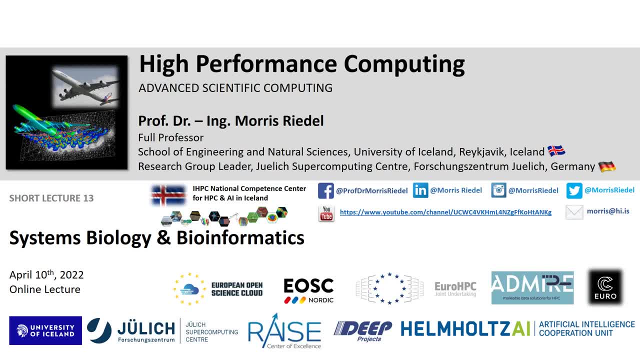 for instance from Paul Malstead, one of the courses in the lecture series that we already started with, essentially with short lecture, 11 with 12, basically on CFD, on health applications, really to understand where HPC makes a difference and area. Of course all of those will have in one way or another benefits of using HPC And that 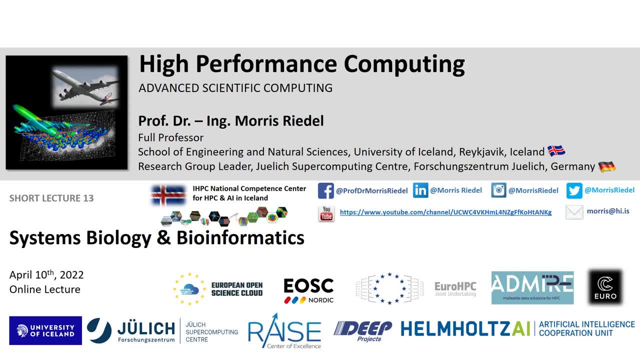 is the idea of basically the short lectures giving you pointers, giving you the relevance of HPC in all the different domains. And with this we start a little bit with a recap that we had the last time. If you remember, my PhD student, Reza, was basically introducing you to the very 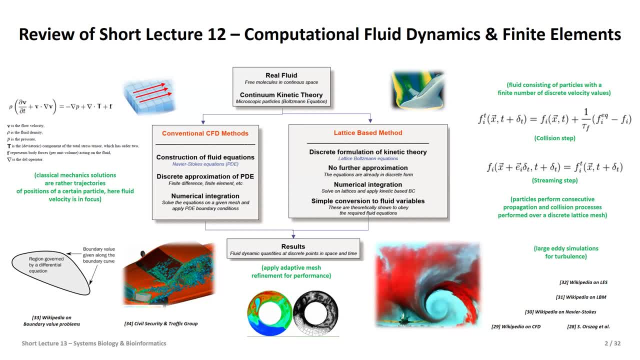 strong HPC user communities in the field of computational fluid dynamics, shortly CFD. That in one way or another also relies on the finite elements methods And there are different schools, so to speak, for different continuum kinetic theory that you see in the idea in the 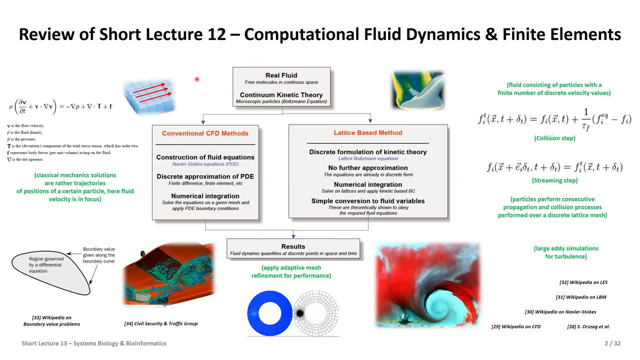 middle to think about real fluid flow basically in the continuous space A little bit. when you think about what we had with our assignment, with the water and wave propagation here, if you want to do it really right, there are kind of two different approaches. 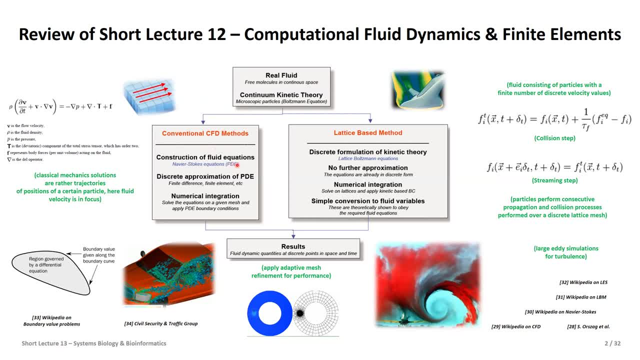 And one would be the conventional CFD method, which is then based on this Navier-Stokes equations, And this is something that also Reza was already alluding to- the role of this partial differential equation. So, basically, the change over time to really find the next evolution of the system. 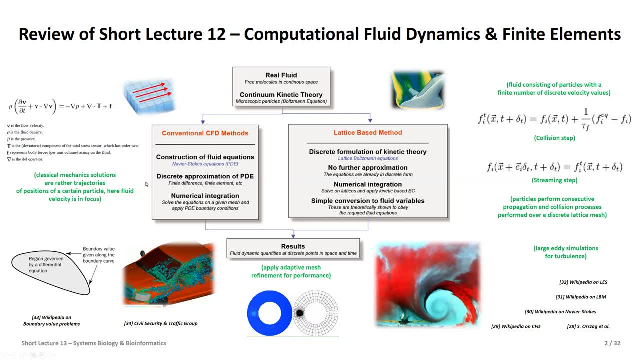 like the whole different loops that we had already in our assignment, with the water waves propagating in the loop from tile to tile. Of course, here you would also think about the fluid equations. so really proper physics over time to really make a real, or let's say approximate a real system. 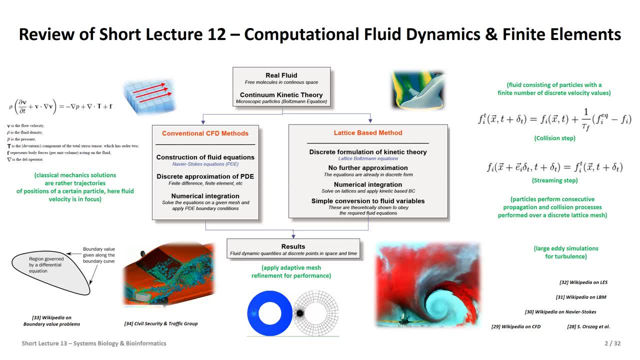 or a real fluid flow, And there are different ways how you do this. We need difference, We need the elements. Basically, Reza has shown light on lots of these different solutions, which are, here and there, rather trajectories of positions in certain particle fields And, of course, here as an example. 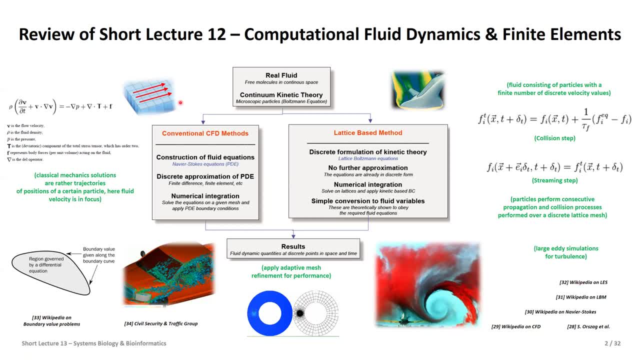 would be the fluid flow that we had in our assignment- want to do it really right- or that also Reza here and there showed, always highlighting the PDEs and also their boundary conditions. so basically, the relevance of saying we have a certain field that we want to simulate and, of course there the boundary values and this would be a 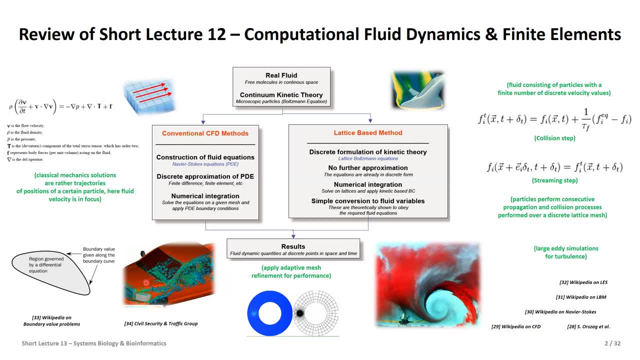 very important part of it, but we have seen that this could also lead to really interesting applications, like here you see, the fluid, basically, or the airflow around, basically one car in the design and development process, or that you see here a little bit with a very specific technique. 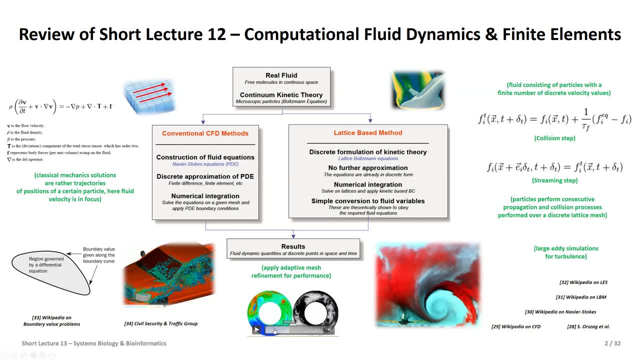 called adaptive mesh refinements, the evolution of smoke in this space over time. so you see here clearly smoke and the fire. and then you see here how in a tube, more like a ring system, here a little bit artificial- that the mesh is refined. and if you want to simulate now how the smoke, 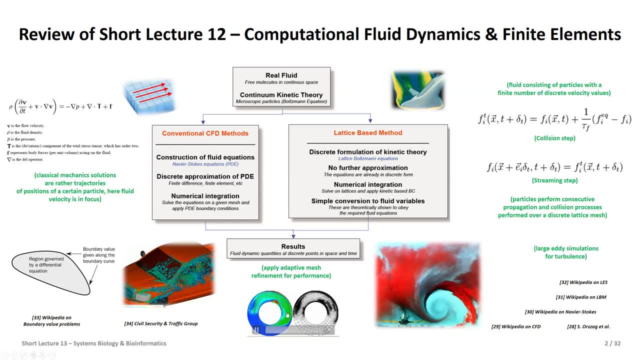 here, for instance, is propagated through this tunnel. you have really good mechanisms in place in HPC based on physical laws, numerical simulations, to really make that happening, and you see here also the mesh which brings us also to this finite element idea of the finite element methods and the meshing basis that we have is basically another part of the approach just wanted. 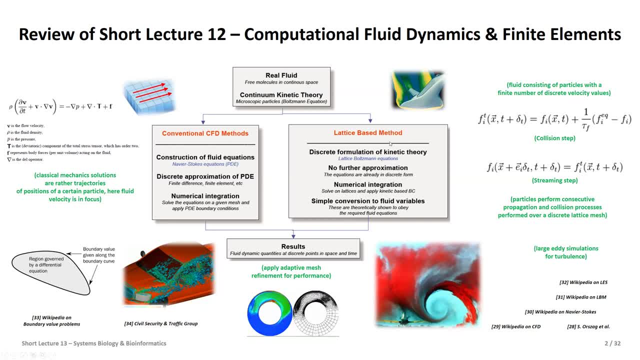 to also bring you the lattice-based method shortly into mind, which is sort of another school on how to do the fluid flow, which is sort of what we're going to be talking about in the next slides: much more lattice, Boltzmann equations about kinetic theory and basically there's also an 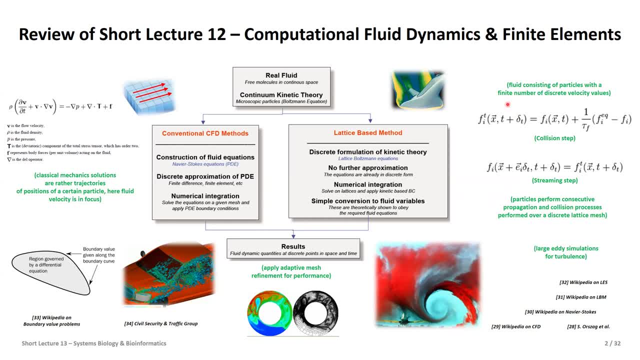 idea of numerical integration based on these, and you see that a little bit here, that you have essentially particles with the finite number of velocity values and there are certain, let's say yeah, equations really that you know give you the collision step, the streaming step, and then, of course, again in a sort of same way that we see. 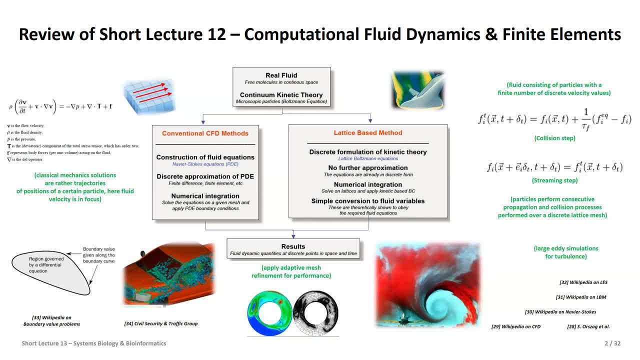 assignment over time. in this loop simulation, we also see how the particles then, in this particular, yeah, fluid flow, or whatever it is what you do, will really, you know, propagate throughout the space, and including also, of course, collision processes that are basically over this discrete lattice mesh. many of these things have been, of course, then, also demonstrated by 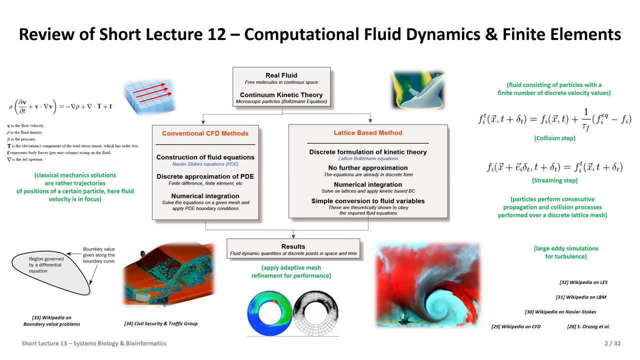 Razor, I think also here. the large eddy simulations for turbulence is also a very good example that you see here from an aircraft. that could be also for different turbulences in water, whatever it is which obstacle is found there. but in the end it shows you that some of these 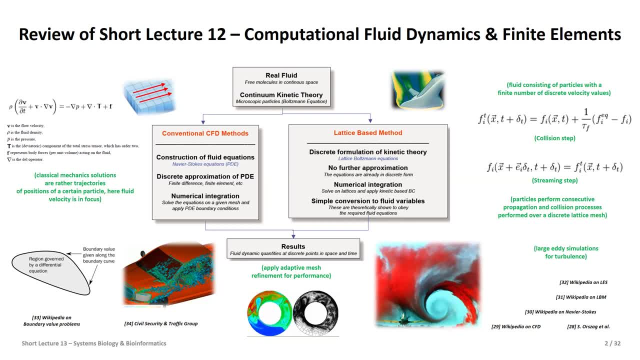 behavior is a little bit like chaotic and also some of these behaviors really require cutting hhpc to really be resolved. and we come to this again today: the idea of thinking about more and more in the second part of the course, about all the different scales and the different 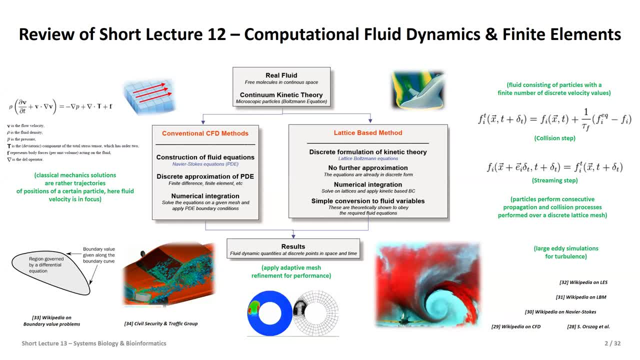 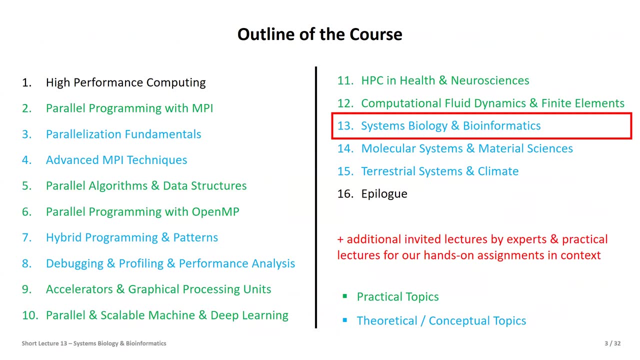 we have the kind of spatial parts that we have, but also temporal scales that we have to really think about. how realistic is it to actually simulate such a system? and today we do this a little bit more on the specific field of systems, biology and bioinformatics. so this is definitely a very broad field where i just give you some 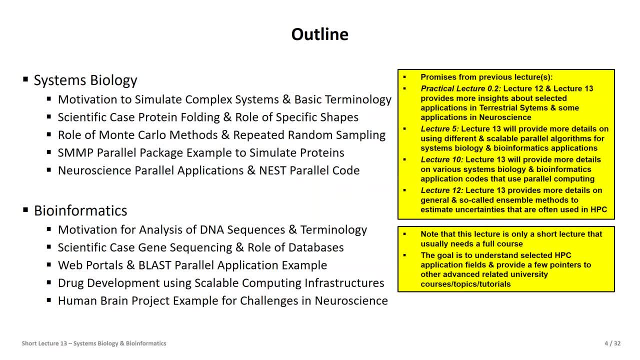 really basic pointers in terms of terminology and what it means to simulate really complex biology systems, and i would pick the one basically here scientific case, which is protein folding, to understand, perhaps with misfoldings here and there, some certain diseases like alzheimer's and so on. so what is the role of a specific shape of a protein? but what i really highlight or want to, 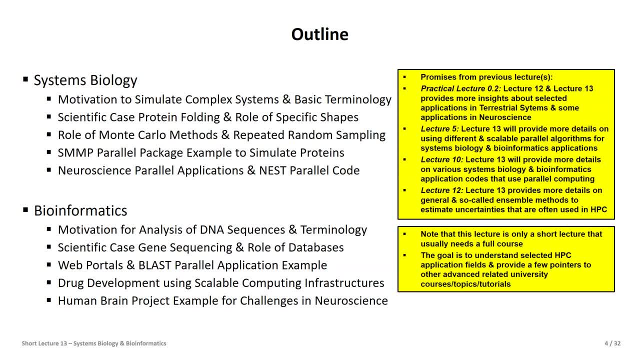 highlight really as part of this hpc lecture. here is then the monte carlo method: right, repeated random sampling. this approach is something which is not at all just for systems biology, but it's basically a very little interesting here to study. but basically you see that it's a general again. 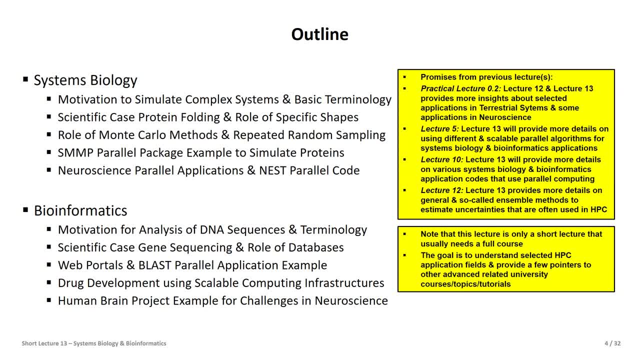 idea of how hpc can be used and the different packages available. here's the ssm, smp package which i would broadly you know, introduce, and also some nest parallel code again. that basically, if you remember, was a bit also linked in shadi's lecture, already in in lecture 11, but the idea 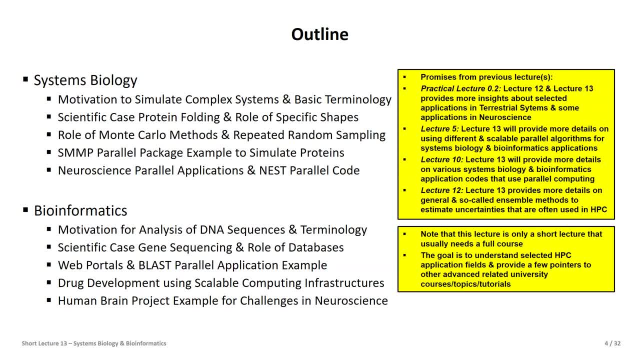 is here really not to be experts in systems biology afterwards. obviously this is a short lecture, so it should also give you really pointers to if that is a field of interest for you- and systems biology is definitely an interesting field, i can tell you. then please use the pointers or do a proper course on that, and the same is actually. 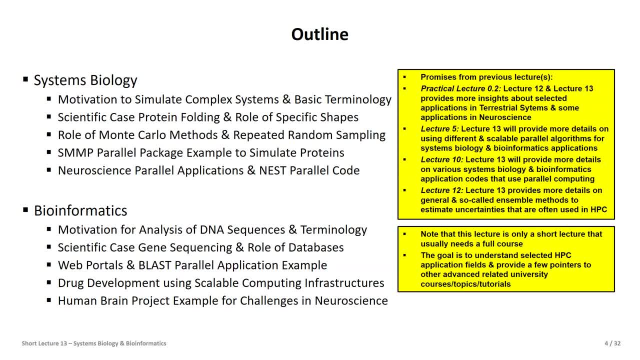 true for bioinformatics. i here just put here one specific aspect, which is perhaps a little bit the idea of the role of databases in this particular- um you know- application scenario of gene sequencing. that i took here as an application example. but obviously the field of bioinformatics is also. 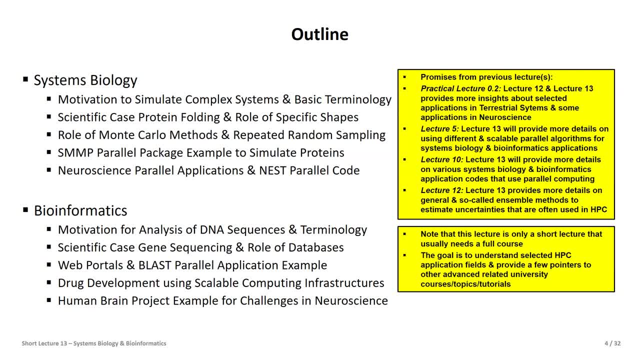 very broad and very important, also having, for instance, drug development, as we saw in one of the- you know- previous lectures as well- already reaching up to a human brain project, and where i also want to give again the challenge of scale for you as an input, why hpc is really. 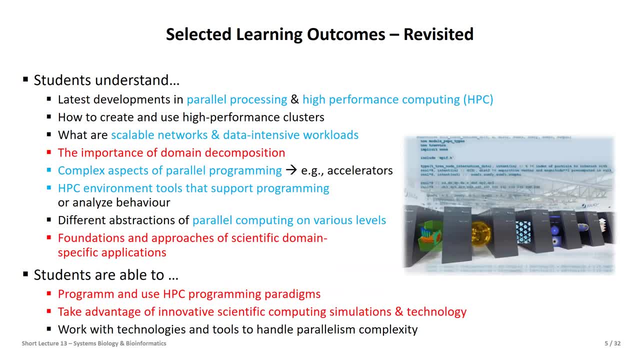 necessary. so what you then really learn from this is more and more the importance of domain decomposition, perhaps not only anymore just on the spatial- you know- decomposition, but also maybe more and more thinking about temporal scales, thinking about scales on different types of atoms, maybe in the- you know- nanometers, up to complete physical structures and engineering of 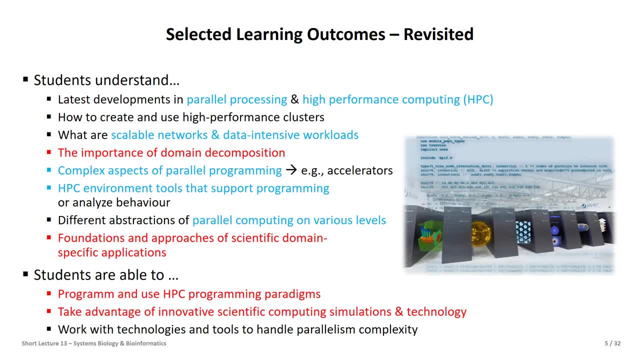 really material products into meters. so you would have a very large range, which we also will basically discuss today and get more and more into the idea how we simulate a real behavior of a system using domain decomposition and then on top of it also of course hpc and with 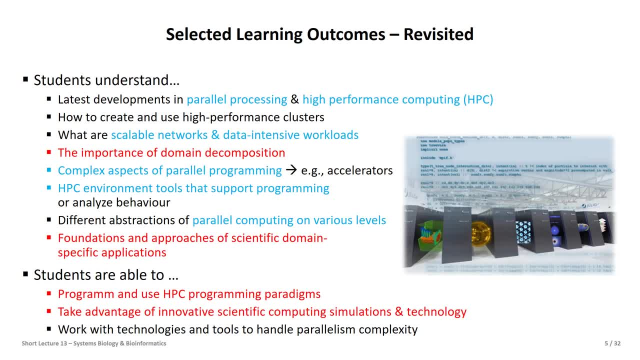 this you really learn another approach for scientific domain, specific applications here based in this one, for instance monte carlo, and then of course very much related methods like protein folding is a big part in hpc in this particular area. and also of course the databases in bioinformatics are very important- the human genome database i will allude to. so let's start a. 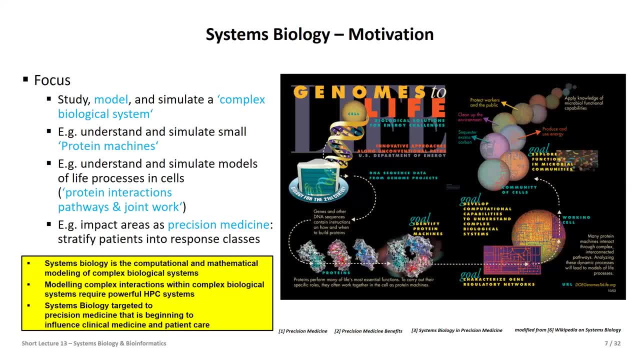 little bit, a bit, you know, basically thinking about systems, biology, and here, of course, the motivation you can imagine is that we have the whole- um, you know, ingredients of us, so that we basically understand a little bit how we actually work as humans and we want to model and basically 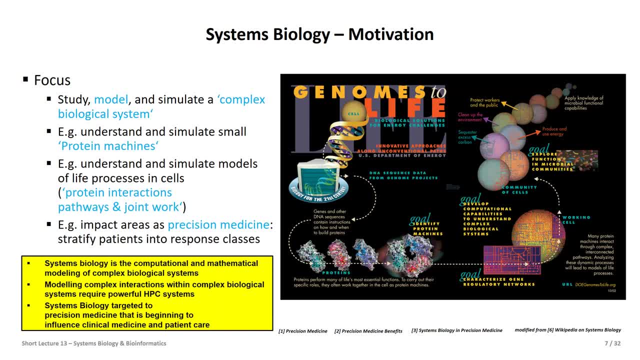 simulate a complex biological systems which could be, for instance, you know, understanding how proteins really work. um, proteins in the body basically derived here from this dna that you probably know a little bit about it. this is you know sequences here that then basically build together can kind of instructions how you create proteins and they are really the. 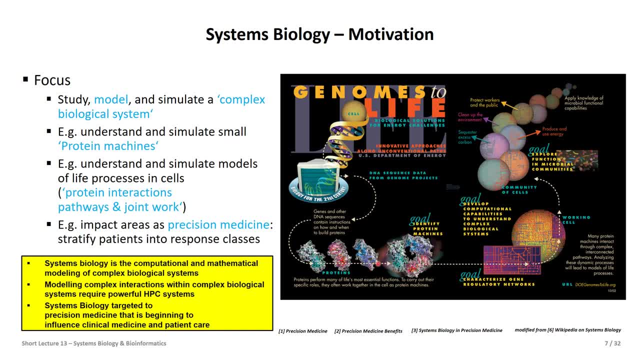 heart, let's say working horses in our bodies, because they really, you know, going towards, you know helping us in terms of fighting diseases and so on. so, in a way, you have something again from different orders of scale, if you think about gene sequences on the one hand, and 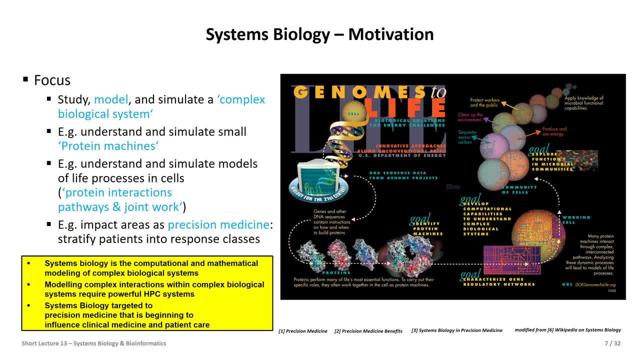 the full folding of proteins. they fall to specific structures and then they have essential functions that we want to study and of course, now, thinking at the end of the scale, you would say we don't want to have this as generally for humans understood. we maybe want to go to something. 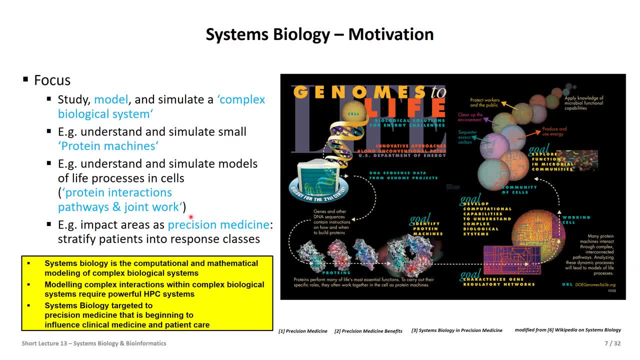 called precision medicine. so this is a field which is also very interesting because there you really stratify- which is a fancy word of saying grouping patients into different response classes, let's say, if it's about medicine, so that you really basically understood that patient groups are different depending on, maybe, their origin in countries, or basically also their age and so on. so 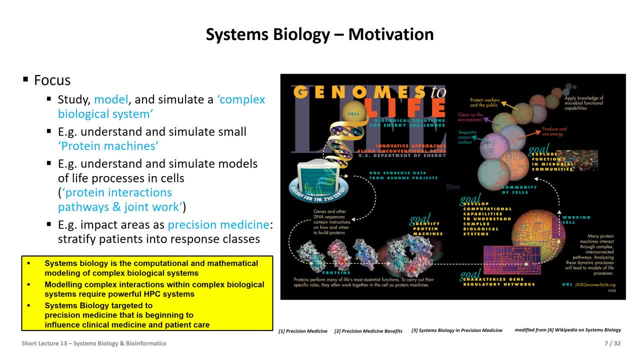 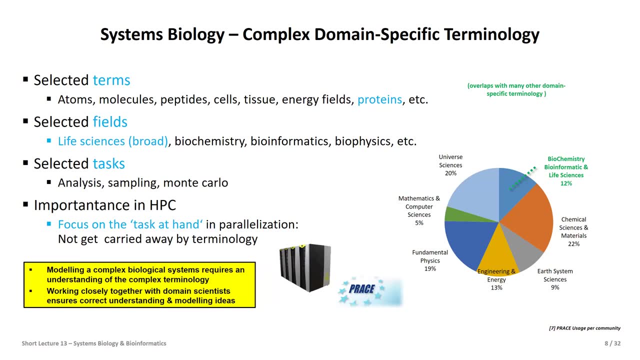 you cannot just generalize very much of saying this is in generally good for the human here. you really want to understand subgroups of us, to really understand and study these responses. so with this goes a little bit short input into different terms of course: atoms, molecules, peptides and so on, and proteins is 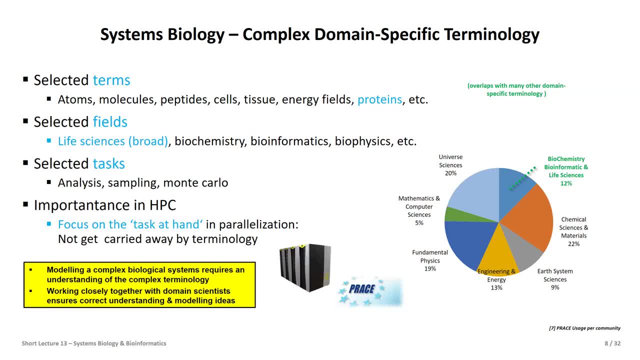 what we cover today a little bit, but all of them is in one way or another related, and we will come back to atoms and molecules also in the next lecture. for instance- and here, um, i would say the field very broadly selected- could you consider here in this lecture as life sciences, which are 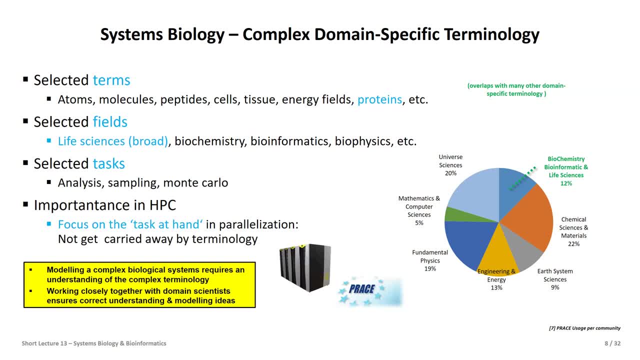 related to this, but also biochemistry, bioinformatics, biophysics- that really understand, then, the law of life and how the way of life is realized in this kind of biological systems. and if you go look and analyze how much systems usage there is in terms of large hpc systems in praise, you can say that 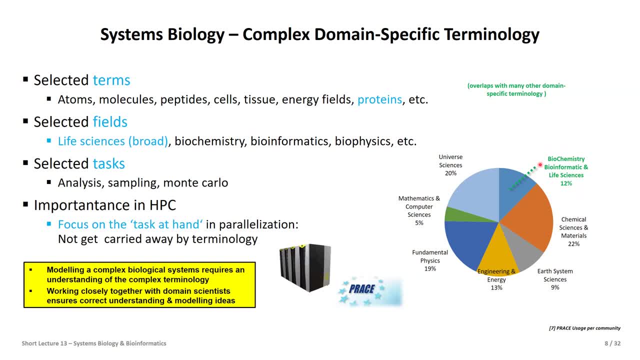 life sciences are quite- it's 12- quite using the systems to a significant degree across, of course, many other sciences which are having, let's say, applications in different areas, also in physics or machine learning, here and there and here a little bit. is this analysis in terms of data and in terms of, basically, the idea of doing the? 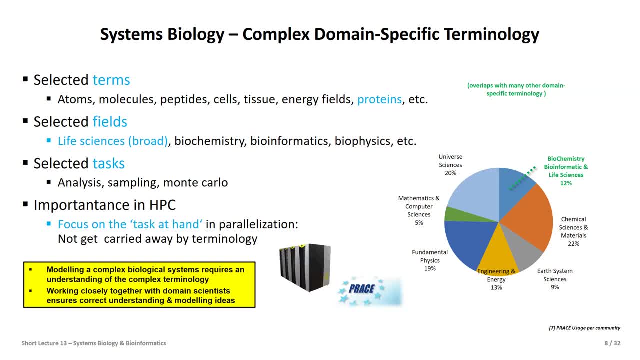 sampling and Monte Carlo methods- I will come to it- And of course there are many of these. basically, you know terminologies, which you then also need, but you also have to collaborate, perhaps with scientific domain experts in the future, if you are an HPC experts. And with this 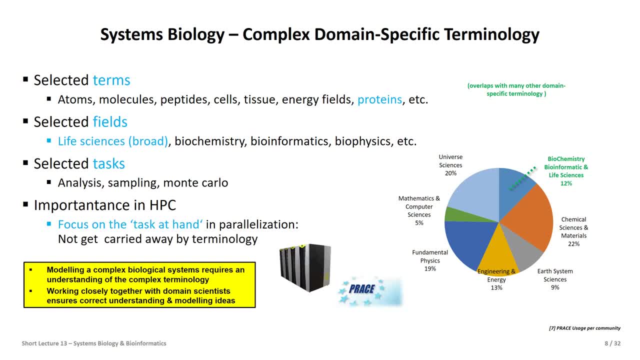 don't carry it away by this terminology. It's, of course, something which correct understanding is best understood. working in teams together, Again as HPC experts, you know you basically also, on the other hand perhaps then a biology expert, then on the other hand also AI experts, more and more. 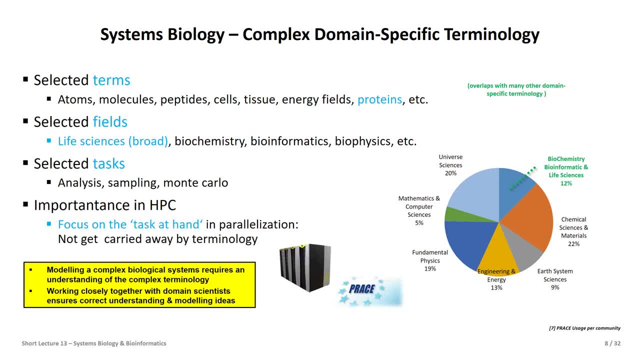 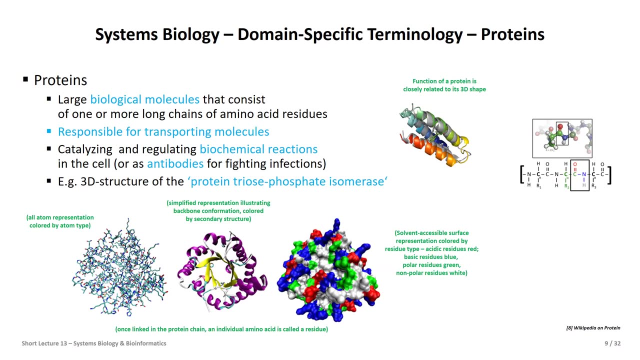 we feel that this is overloading people, So it's much more realistic to think about working in smaller teams to really get today the best out of systems, biology and many other applications. So this domain specific terminology in terms of proteins. I already was saying they basically 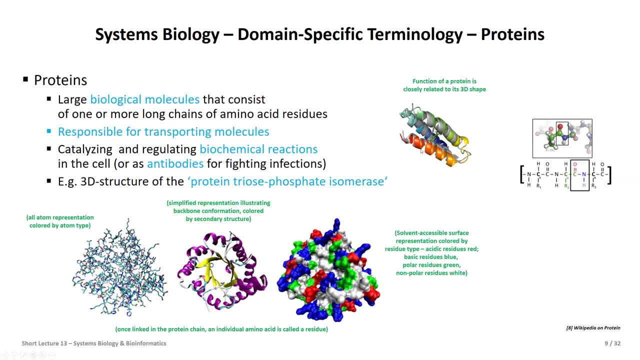 derive from what we know, we see, basically DNA, and then they have a very, you know, kind of specific 3D structure. they can take again and again in order to do a particular function in the human body And of course, there are different areas of scale. again, how you can actually do this. 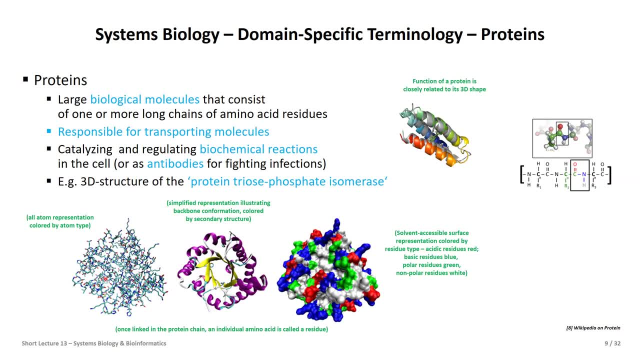 So you see, here is all atom representation, which is really then going into the atom type of presentation. then you have this kind of secondary structure which is a little bit more, let's say, simpler, and then basically a very specific structure here, which you have them called a. so 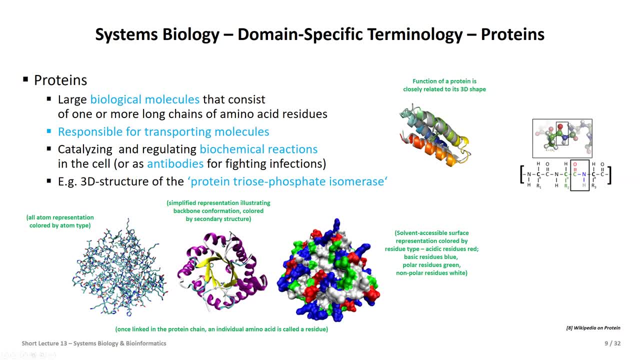 called, yeah, residue Again, this will be lots of kind of terminology, just to say the basic idea of you know how this basically works in all you can think about that. of course these atoms will have force fields. they basically can be, as we see later here. you know, basically form proteins in. 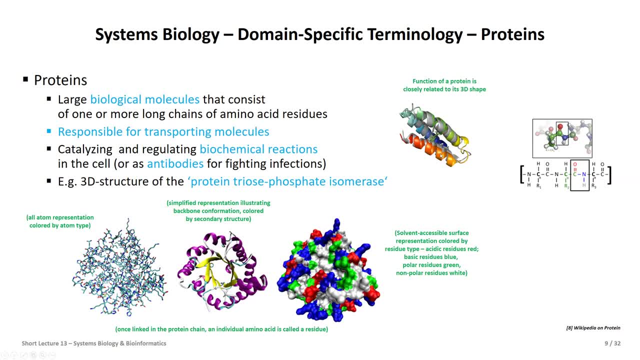 different structures And this is something which, in the end, you know, goes back again, on different orders of scale, then to long chains of these amino acids that we know, but, of course, then being in some form or another when they do. 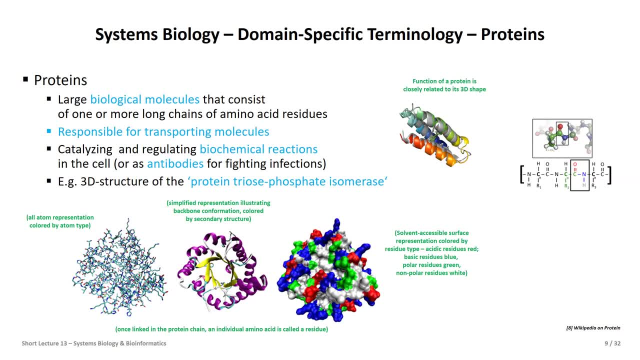 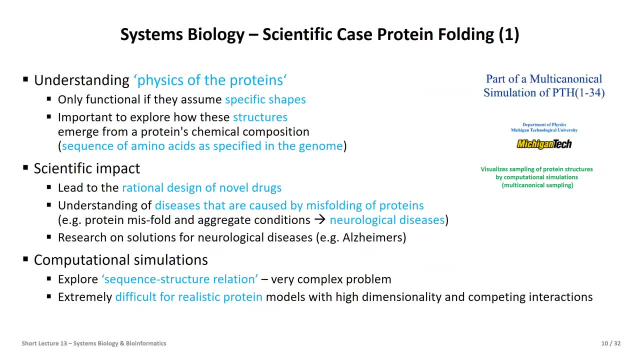 for instance, a specific 3d structure, then basically fighting specific infections in your body. So in the end, of course, you have to study this material much more into detail if you want to become an expert in systems biology. Here's an example of all this different, you know. 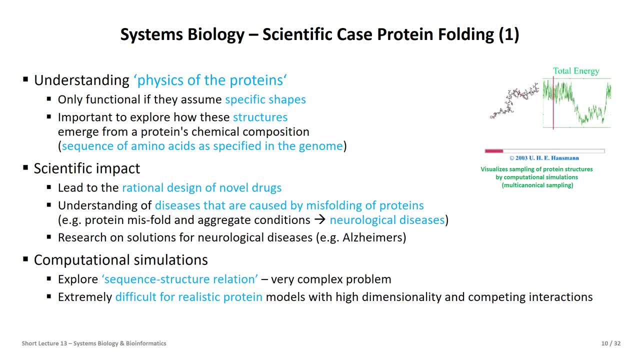 variations and sampling of protein structures, where you basically use now HPC to sample all of these different protein structures, because this amino acids that we had described and the structure and to really form the specific shapes. it's not at all very clear, right? So, basically, this is what you want. 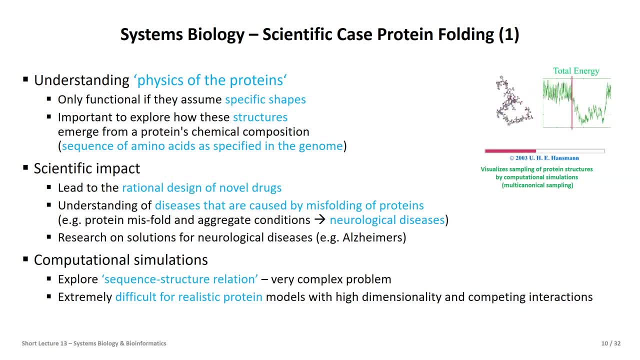 to understand, in particular in the light of the fact that basically some of the misfoldings of these proteins happening in the human body are actually known to actually get, with aggregate conditions, to neurological diseases like Alzheimer's. basically, that is perhaps related to this And of course it is, you know, basically computational simulations. 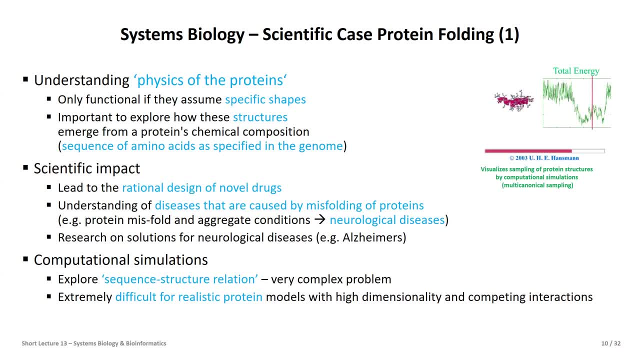 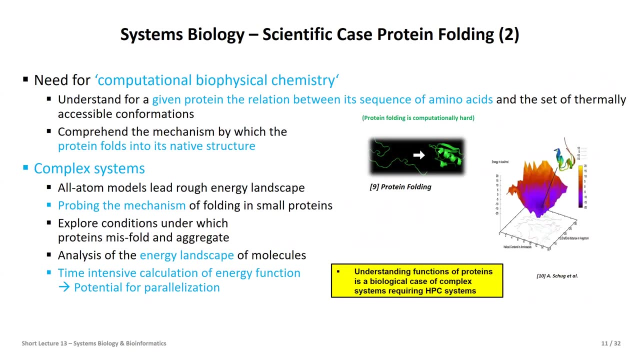 very compute, intensive to do so. hence the case for HPC is made, And this is a very interesting 3d sequence structure relation problem of forming this folding So very complex problem really requiring loads of magnitudes of scale And then also, of course, lots of different approaches to 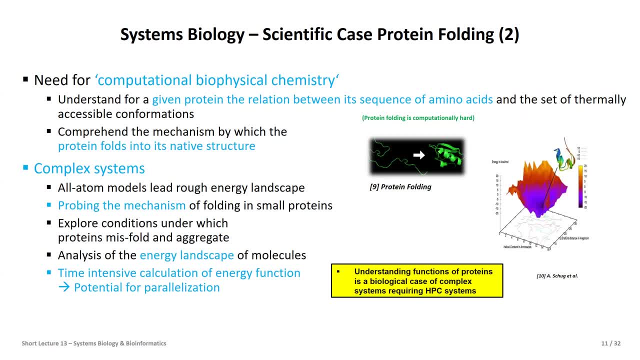 find specific 3d structures. So the idea is: and really, given you have this protein, the relationship and the sequence of amino acids, which basically is of course clear, then we basically think about, we have this long line that 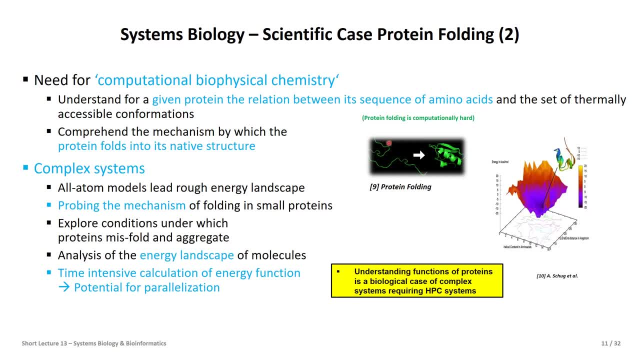 you see a little bit here alluding to in this and depending on what now is basically happening with the body, obviously, let's say external stimulus- we want to understand really the function of the protein. then in of a complex system. what's happening when i perhaps then do the 3d fold that i described? 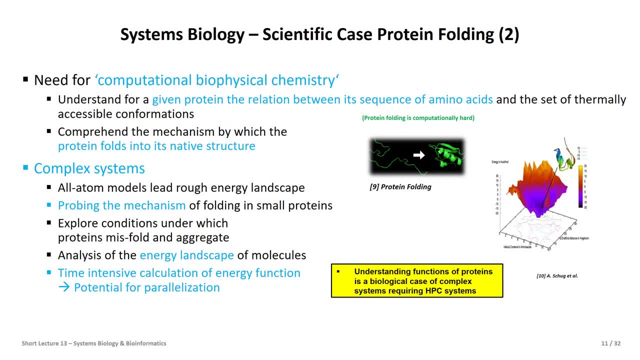 and then you have different conditions, very many um, and of course, when you have this, all atom models that we had on the other slide, um, then basically have a very interesting- you know, energy landscape of thinking how well is the structure formed? um, you basically have then interesting. 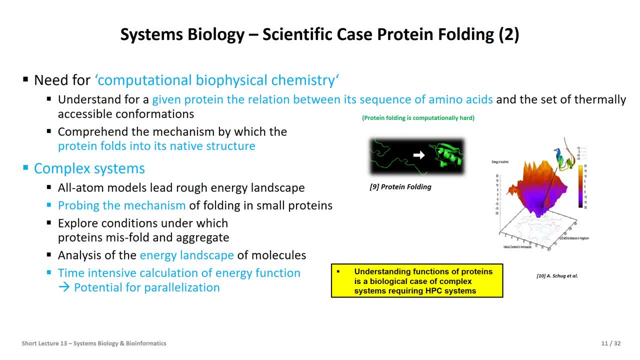 conditions, which you can study by using energy functions and so on, and all of these time intensive calculations then make up the idea of doing this perhaps in parallel, using parallelization. that we've seen already from the sansman group in the previous example, so really want to understand the function of proteins. here's another one of these examples. 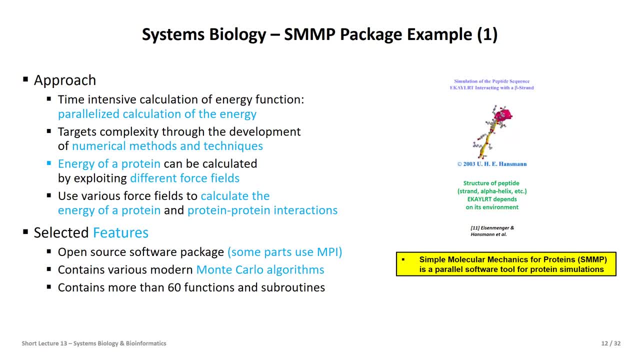 as i said, to really find essentially the, the different, um, you know proteins and they have then been they found and basically, if you have used tools like here, the simple molecular mechanics for proteins, tools, which is really then a parallelization of these approaches for protein simulations, then you basically find specific structure and found, let's say, an. 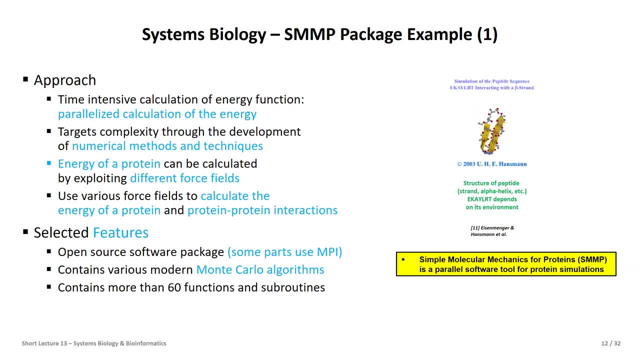 interesting part in system biology that you can publish, that you can contribute to the really complex area of systems biology that we will look into much more. coming back to the energy function, of course you think about that. all um of these approaches that we have um basically need to be under the 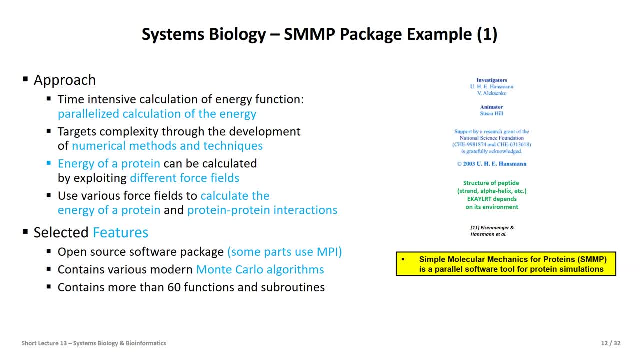 rules of physics. so there are different equations that you have to adhere to, but we have numerical methods and techniques to do this then over time, because there's not this one solution directly that you can, let's say, compute the closed form solution and some people would say just directly. 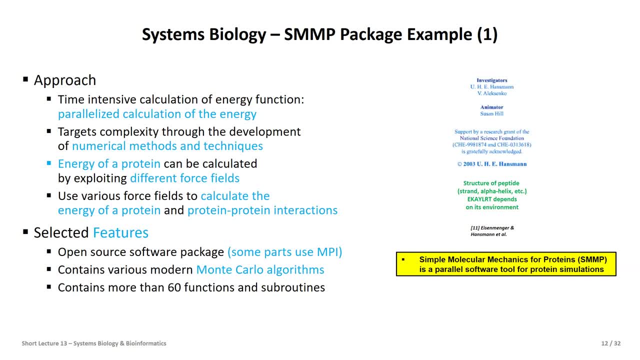 solving everything. so you go with this numerical, iterative approaches to basically calculate, then, the energy of proteins, and of course this is related to different force fields also. thinking about that, all in the end are atoms that are interacting with each other, and we will come to this again and again when we basically go through the course here today, in lecture 30, but also. 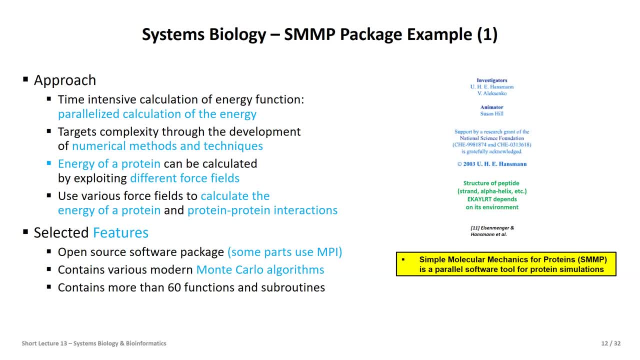 lecture 14 will actually reflect on these parts. and to come back to the initial part of the lecture, smmp, it leverages of course some parts of mpi. so you see that mpi is relevant also here in the systems biology domain, in particular light of the fact of this code here. but of course, 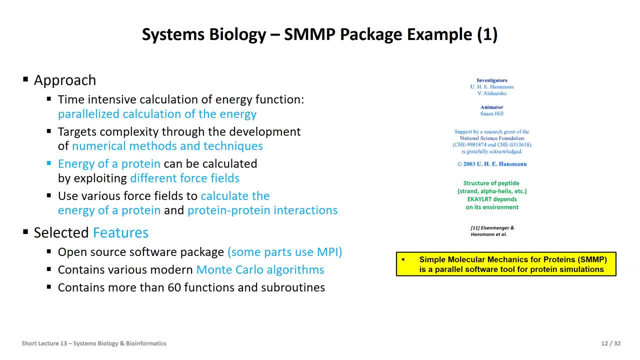 of many others also, and here um some of these pictures of these kind of features that we want to highlight here is now this monte carlo algorithm. i want to point to a little bit this repeated random sampling, which makes sense in some application areas, including here this. 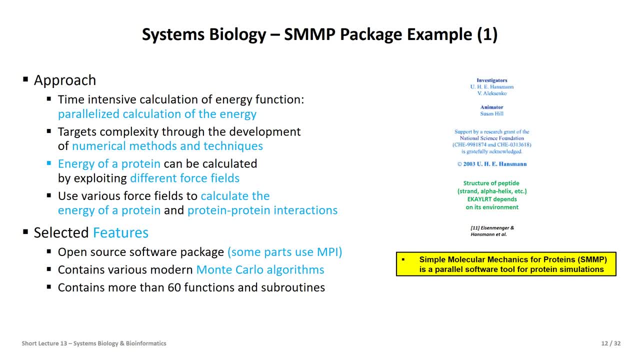 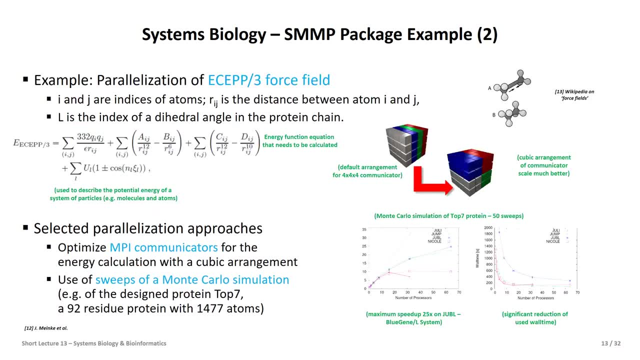 protein folding. but of course, if you look broader, the smmp, mps package, as around 60 functions and more in its subroutines. so also what you can see there is it reuses really elements that you know from previous lectures: mpi communicators for energy. 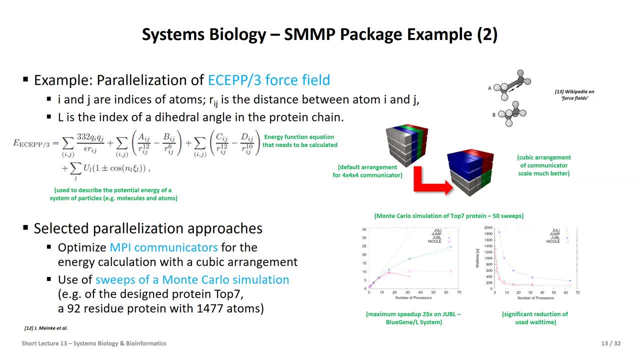 calculations and here with the kubrick arrangements, which we also had discussed in one of our previous, let's say more theoretical aspects or conceptual ideas, that it really depends how you structure your domain. decomposition: here is a very important example again where you see the color coding of the parallelization. 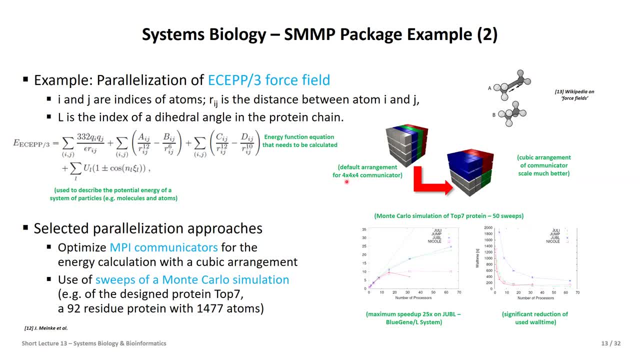 strategy, which is here the default arrangement. for instance, if you do four times four times four. but here we really can see that if you do a cubic arrangement, then we can see that the scaling is much better and we had already seen in one of our lectures that of course the communication. 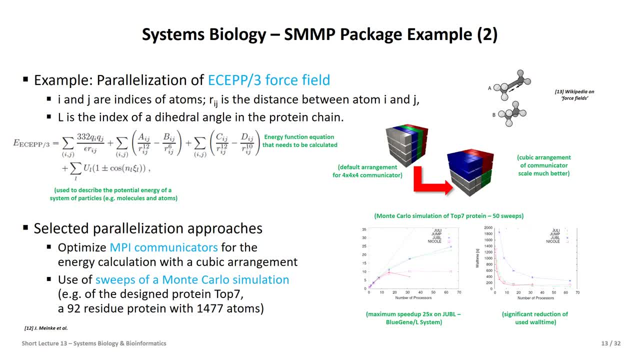 is less here, so it scales much better. and if you do a monte carlo simulation of the so-called top 7 and do maybe 50 sweeps, you see here a little bit different hpc systems and their scaling behavior, um where basically you see also that not all of these approaches scale on different systems. 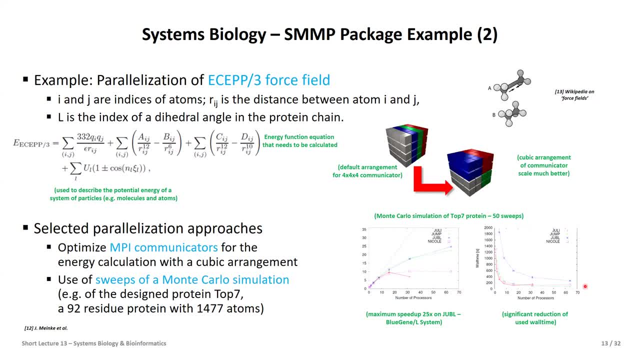 but in the end we see, with already scaling up to more and more processors, we can here reduce the, let's say, time to solution in the end. still, we want to understand what means sweeps of a monte carlo simulation. we have a specific protein i want to study. um, i know a little bit about it so, and i have here. 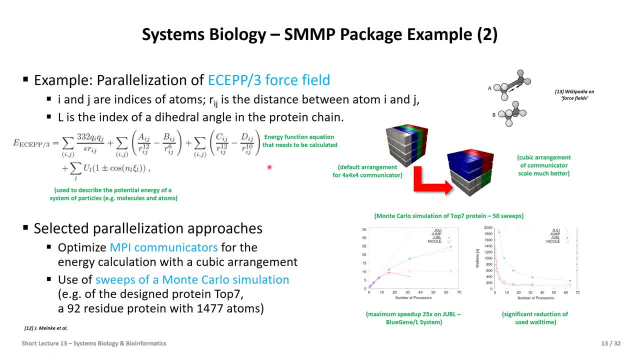 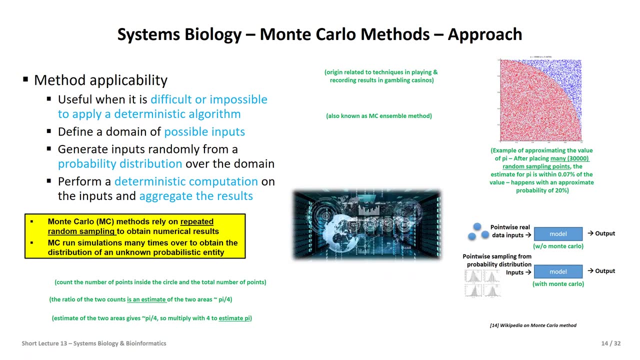 this kind of force field, id, and, as i said, also there are specific laws of physics that you can then use to have the energy functions calculated with hpc and of course then these kind of tools like smmp i was alluding to. but monte carlo then really means, as the overall approach is, that it's. 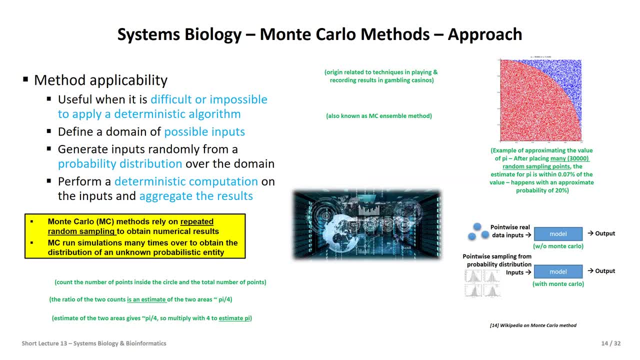 really applicable? if there's. it's basically impossible to do a deterministic algorithm, so you need basically to define a possible input domain and this is something where usually there's a good example of thinking about this calculation of p that is here essentially nicely visualized so you can approximate the example of p or the value of p, really of doing this repeated random sample. 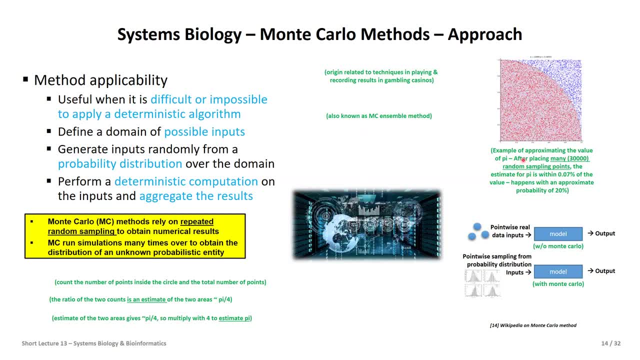 and d is the idea is not doing it once or twice here. if you do, after placing many, let's say 30 000- right points here, then you basically can estimate p actually within 0.07 percent of the value. so that is quite good. of course, this is a probabilistic assumption. again, how, depending how, 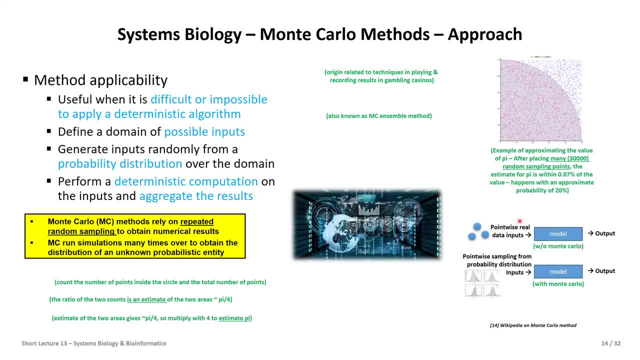 often you do the experiment and this is something when you calculated a little bit and the results of this. so the point-wise data inputs that you have, which give you the model then and gives you then, of course, then the output without monte carlo. but if you do it basically with real data inputs, it can be very many or you just have not enough. 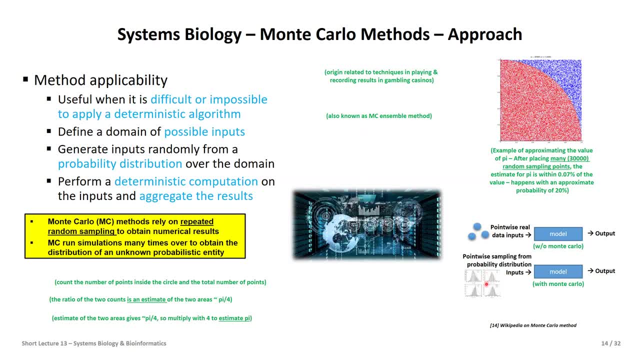 representatives of those. so you do a kind of point-wise sampling of the probability distribution behind the inputs and with this iteratively- which we say this is repeated random sampling, you have this kind of so-called numerical results using this monte carlo method which works here for 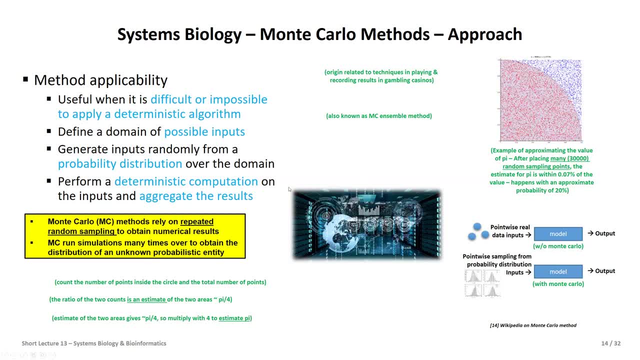 p but also works basically, then if you translate it again to the protein folding idea of many different possibilities, but then you basically do a sampling of all of these probability inputs and come to this over time of course, then to a numerical solution or a numerical result and this overall approach by really running the simulations very many times with hpc. then you 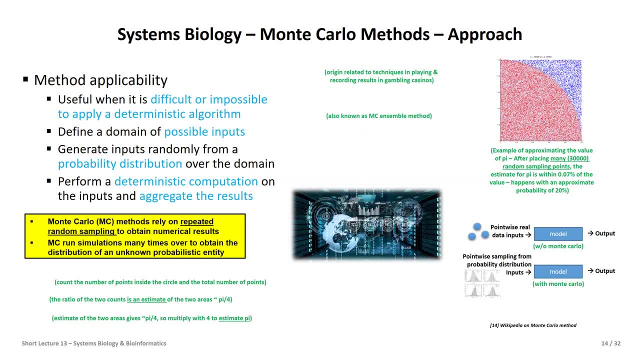 basically obtain the distribution of this unknown a probabilistic entity that you have. this is called. sometimes also people say monte carlo ensemble method, because you're not running monte carlo once or twice. it doesn't make sense for monte carlo, as the name suggests, in a gambling casino. 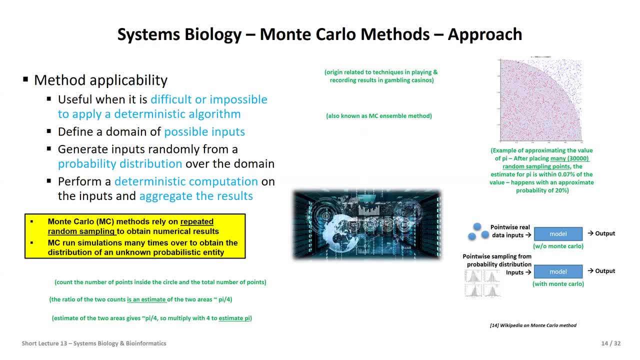 right, in order to win, you really have to do a lot of playing to do this, and how it works exactly. um, basically, you see here a little bit alluded: you have the points inside the circle and the total number of points you drop in the space, and then the ratio of these two is an estimate of the two. 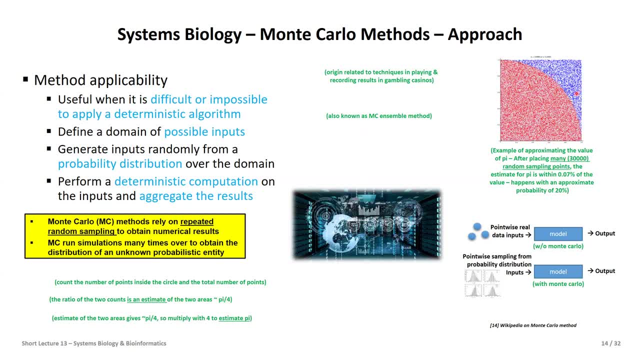 areas, which is of course obviously p divided by four, and then you this two areas estimation is of course. then multiply it with four, because we just do it here in this particular area, and then you basically have an estimate of p, and you're just doing this. so 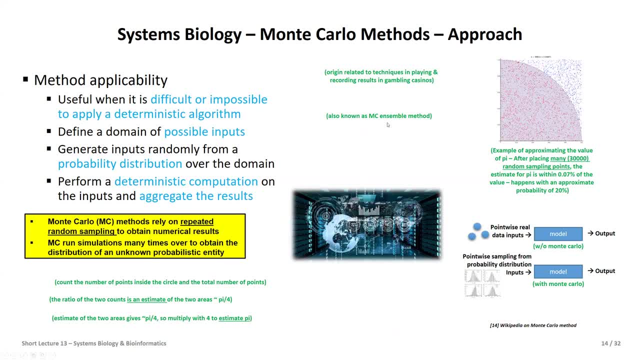 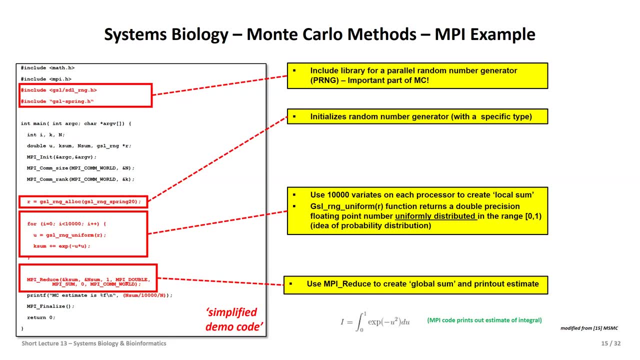 basically by dropping these let's say points again and again in this space, and if you want to program it, here's an example how you would do it. with mpi, you have a specific library called prng. it's basically a random number generator. that can be important, that you, of course, then 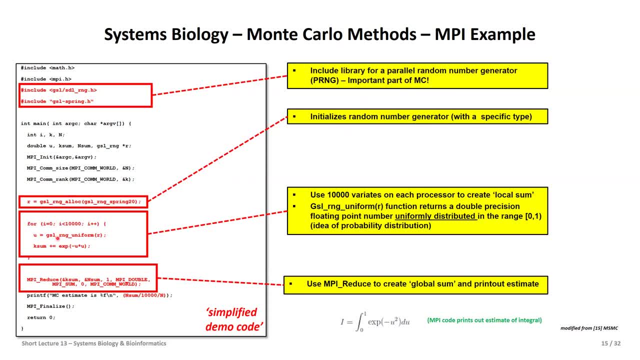 have to. you know, basically um initialize and then you do the loop, as i said before, and here's an example of 10 000 variants right for each of the pro processor that create this local sum. so you do this: 10 000 experiments on each of the different processes. 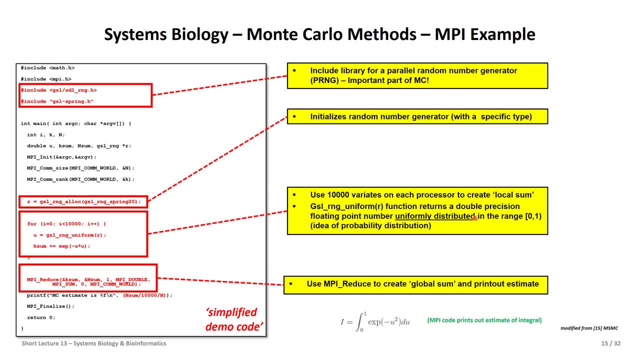 and do then essentially this kind of idea that we had seen with p dropping the points, and once you have done this independently on all the different processors, you collect the results with mpi reduced to create the global sum and then with this, as you remember from the um, you know equations or the description really, before um we can have 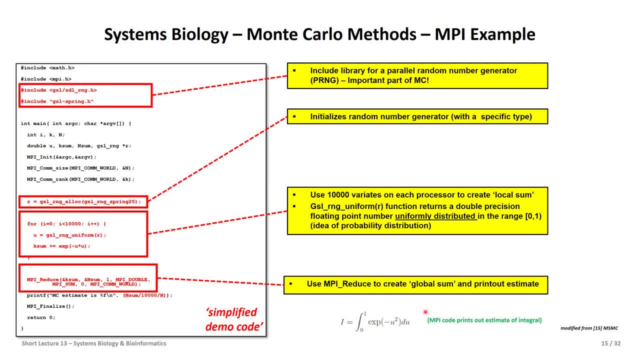 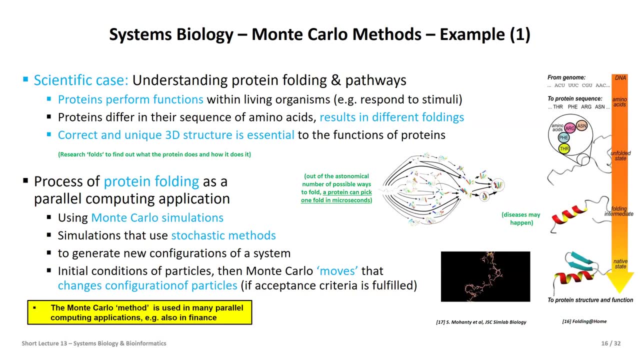 an estimate of this integral that is then responsible to approximate p. so a very, let's say, simple algorithm, a bit simplified even as a demo code for you here, but shows the essence that of course those mechanisms are used in practice, for instance here in the systems biology. 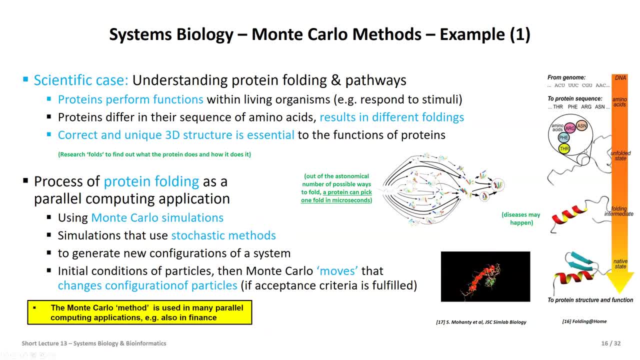 domain, and here you see the complexity of this as well. so we start again from the genome and then we go to different amino acids, as we already know, to this unfolded, long state that i was eluding earlier, which is just this kind of concatenation of amino acids, and then we want: 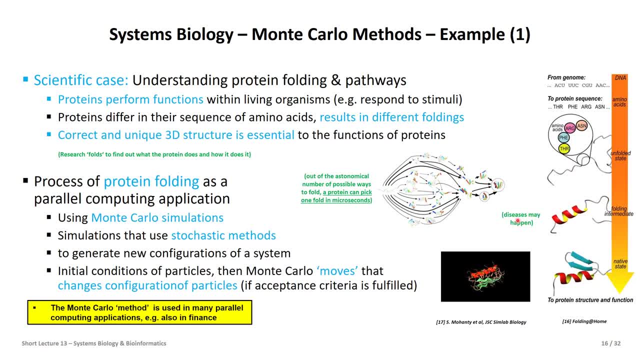 to do this folding and studying, and here's where the diseases may happen. you see that here a little bit here in the time over time simulations, right, how this long string here then again and again gets basically then to a real um, let's say, protein building in this 3d. 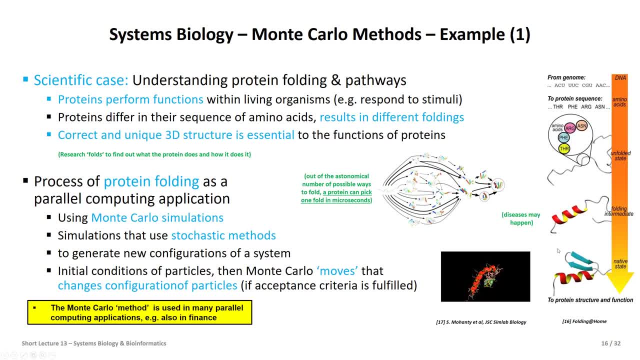 structure and hopefully gets in some native state. but to go there, you see this, astronomical ways, possible, right, in order to achieve that, in order to take the same way, and um, the protein can pick this one fold in microseconds. so we have to understand, really, that this is a. 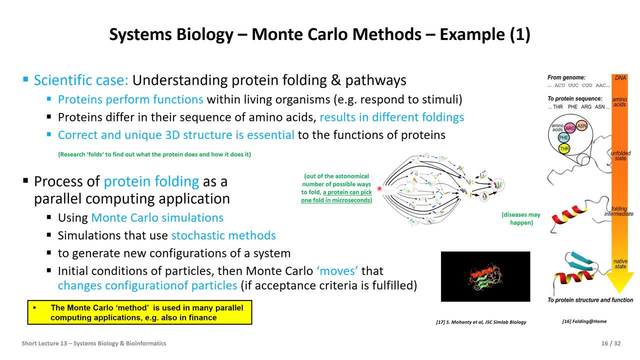 very short time interval that we study here as basically simulation scientists, and here you can use it essentially with the pro, with the monte carlo method, nicely, because all of these pathways, a little bit can be done, let's say, in a no parallel way to understand what would be the best. 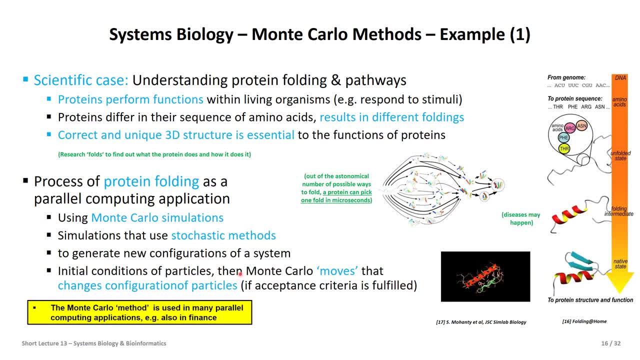 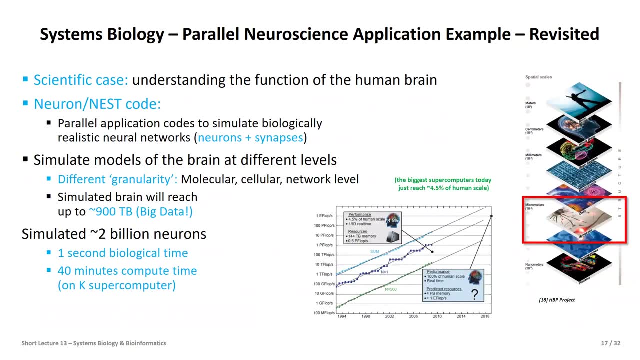 way moving forward. and this monte carlo simulation, just to close a little bit on this. i could talk, of course, long about this. it's used not only basically in biology, it's also used in finance and other hbc areas. now, when you think about systems biology as a whole, of course, think about that. um, here the 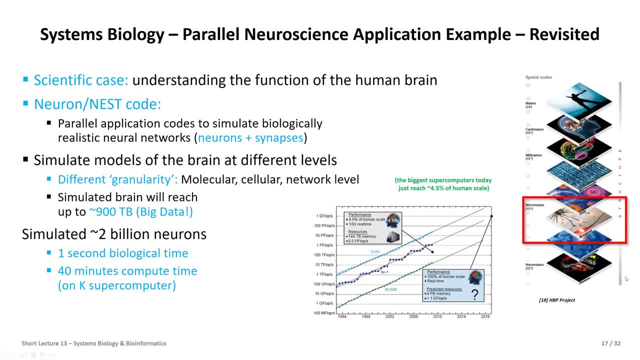 overall approach is really, in the future, thinking about more scales, and i will come back to this again and again when we have our ideas then of the um- you know- lecture as a whole thing about these different scales. here the human brain simulation is just 4.5 percent of the human scale. 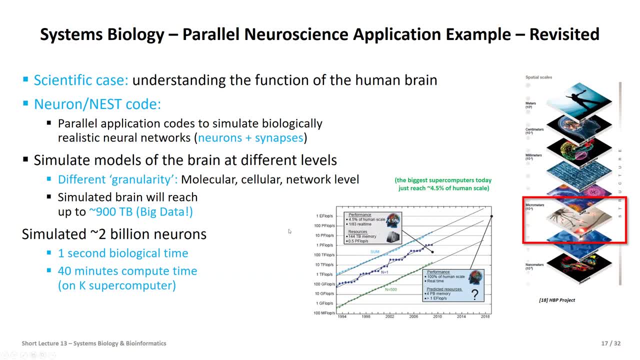 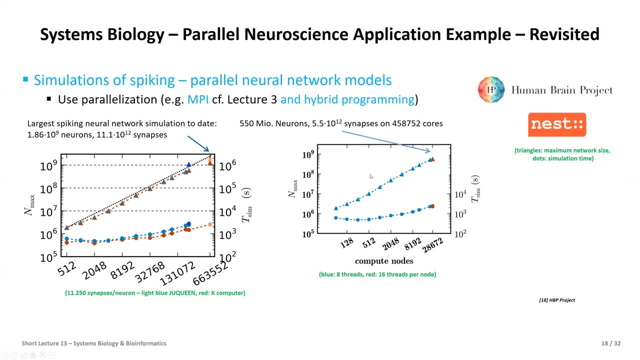 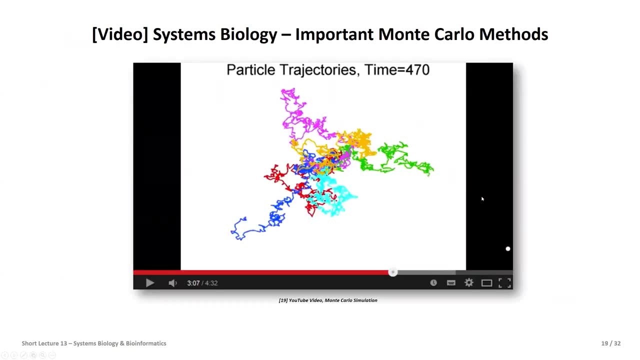 what we already had in one of the other lectures, for example, good, and there's a nest code that basically is able to scale today much higher than i printed here. that is basically also reusing technologies like mpi and hybrid programming, also some code that we already were pointing to. just let us now review a little bit this monte carlo simulations. 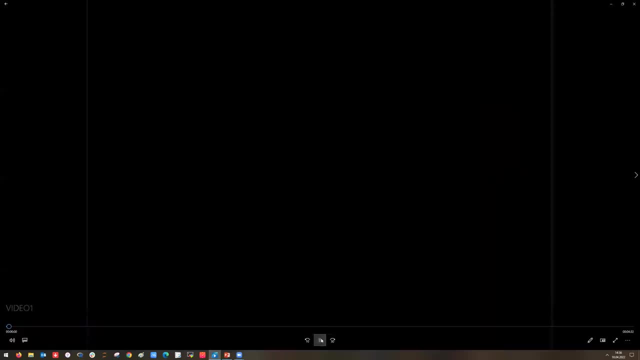 and then as a video before we come to the second part in the short lecture. hey, this is kevin and you're listening to the second episode of kevin's math and science podcast. so today's topic is monte carlo simulations. when trying to define monte carlo simulations, a quote from the supreme 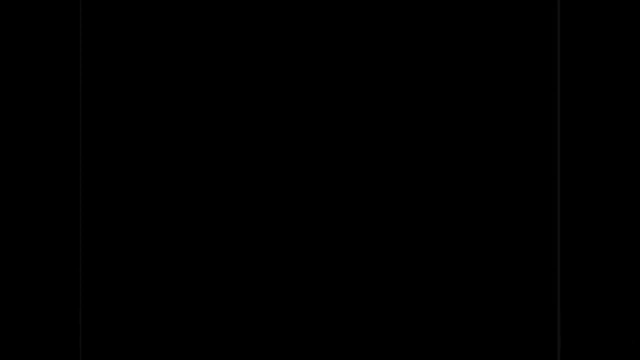 court on pornography came to mind. you know it when you see it. this is because it's hard to find a good definition, but the basic principle of monte carlo simulations is that they use a large amount of random sampling or random tests to find some large aggregate property of the system. let's 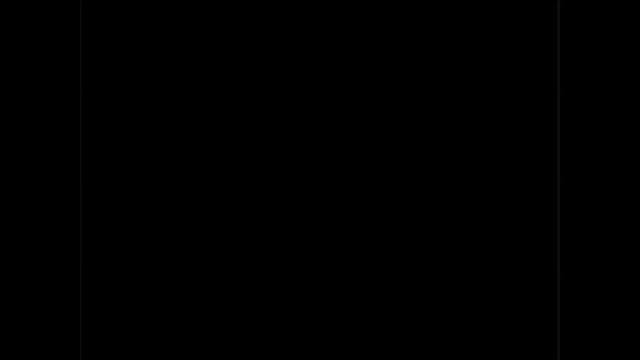 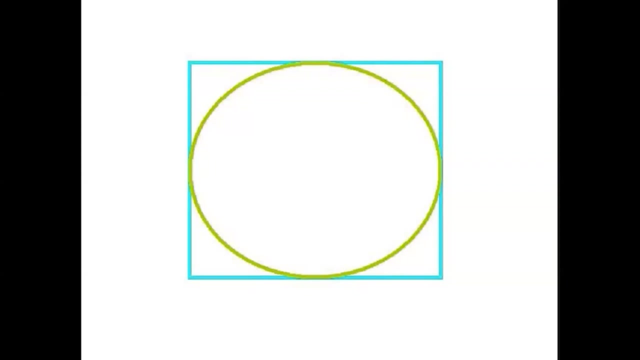 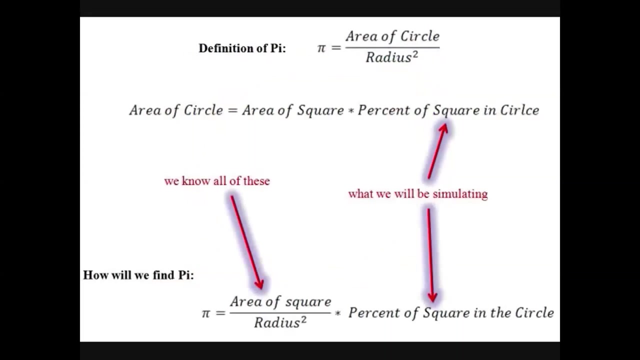 demonstrate a monte carlo simulation by using it to find the value of pi. imagine drawing a circle inscribed in a square. we assume we don't know pi, but we do know two things. then we can use monte carlo methods to solve this problem. the first thing we need to do is to define pi, which, for our purposes, 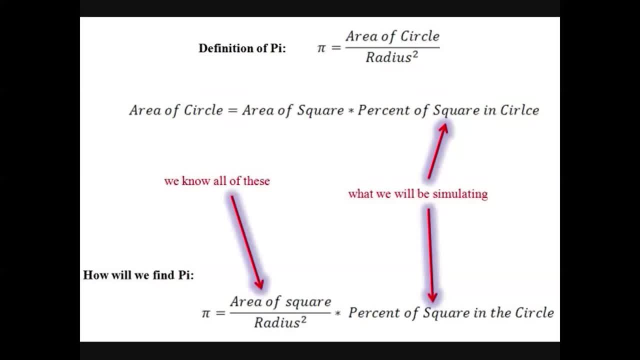 is the ratio of the circle's area to its radius squared. we also know that the circle's area equals the squares area times the percent of the square inside the circle. when we combine these two equations we get the formula for pi at the bottom of the screen, which we will be using for these. 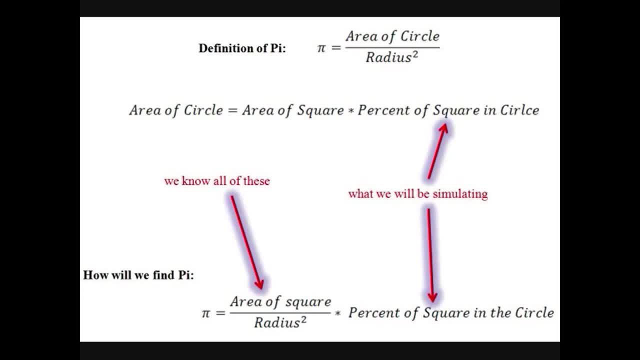 monte carlo simulations notice that we know the radius of the circle and the area of the square since we drew them. we don't know the percent area that the circle occupies in the square, and this is truly the unknown that we will be solving for with the simulation. 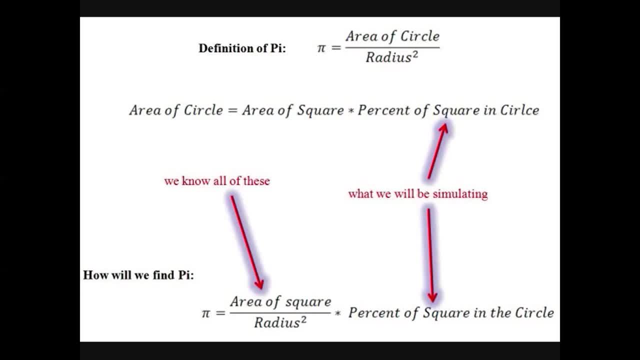 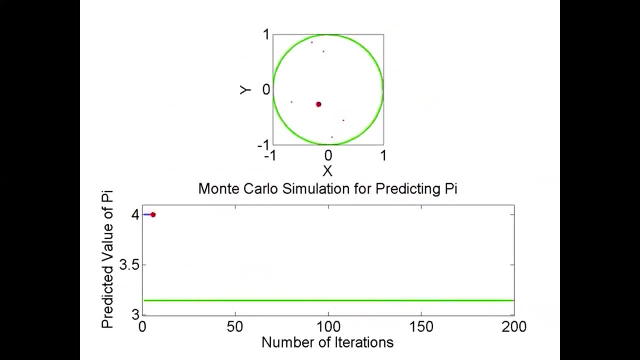 the formula we'll be using for pi is that pi equals the area of the square divided by the radius, squared times the percent of the square's area occupied by the circle. this is what we will actually be simulating to find. we will do the computational equivalent of randomly tossing a. 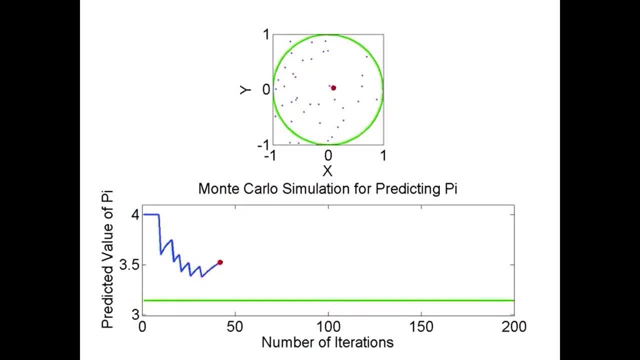 stone into the square. the percent of times that the randomly tossed stone lands in the square approaches the real percent area of the circle, as the number of tosses increases to infinity. this is what you are looking at now. on the top you see a square with the circle inside it in green. 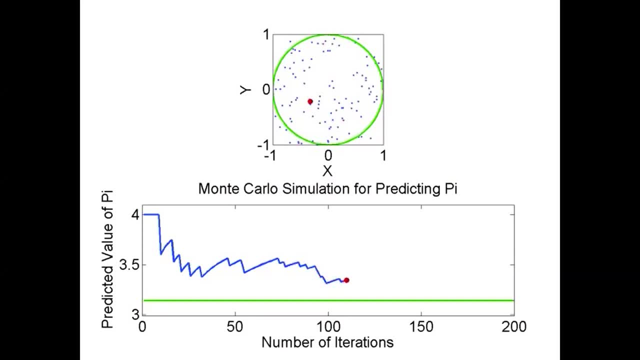 the stone just tossed is in red and all previous tosses are in blue. then on the graph below you see the predicted value of pi as a function of the number of random tosses. the blue line is the predicted value, while the green line is the actual value of pi and the number of random tosses is the. 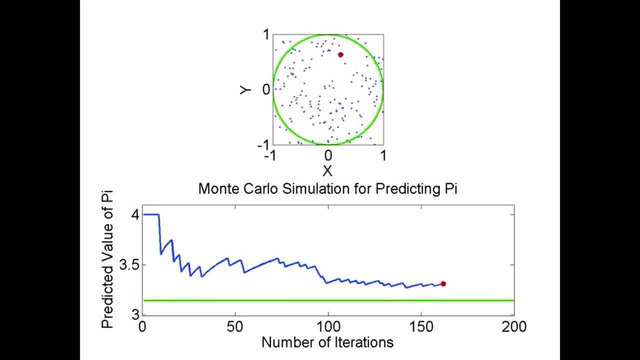 actual value of pi 3.14, etc. notice that at first you start far from the predicted value, slowly moving closer but with large oscillations up and down. eventually you might even reach 3.14, but you'll overshoot and then undershoot because of the oscillations. 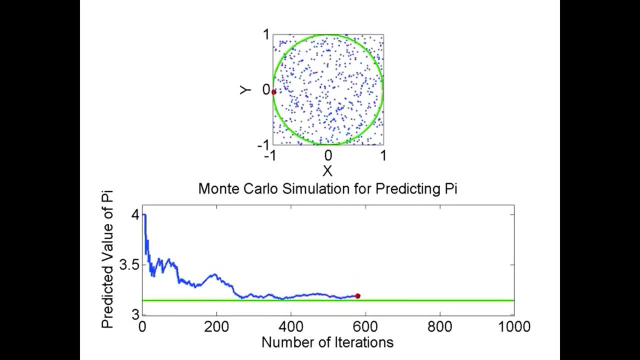 as the number of iterations increases, the oscillations dampen, and by the time you get to 10 000 tosses, the monte carlo simulation seems to be asymptotically approaching the real value of pi. what's so cool is that from completely random tosses we can get a really good estimate of pi. 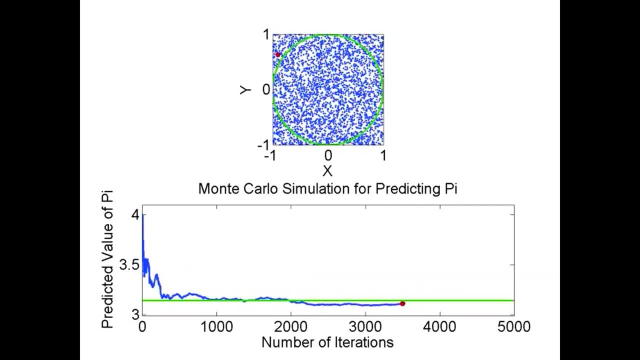 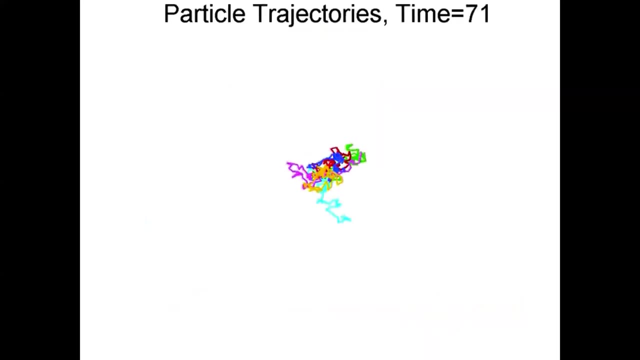 for something random. from something random we can get a deterministic property, in this case pi. another example of monte carlo simulations is what we looked at last week, the brownian motion of particles, remember. we showed five randomly moving or brownian particle trajectories starting at the center, just like when we calculated pi. at only five iterations we don't get any real sense. 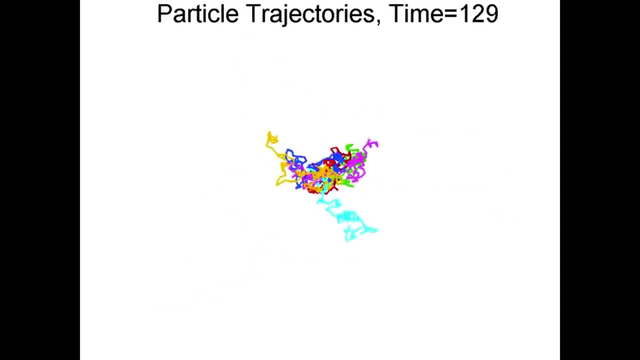 of the information. then when, instead of simulating five particles, we simulate 500, we do see something interesting. we see that random motion looks a lot like diffusion, like a drop of dye into a dish of water, a slow dissipation of gradients as the molecules spread out. this is one way that monte carlo simulations 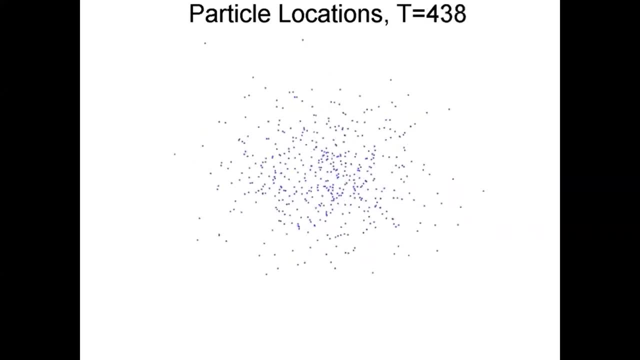 can give us interesting information about particles. we see that when particles move randomly, you get diffusion. monte carlo simulations are used in everything from complex molecular simulations to complex molecular simulations, and molecular simulations to complex molecular simulations, to financial modeling, to understanding how viruses spread. 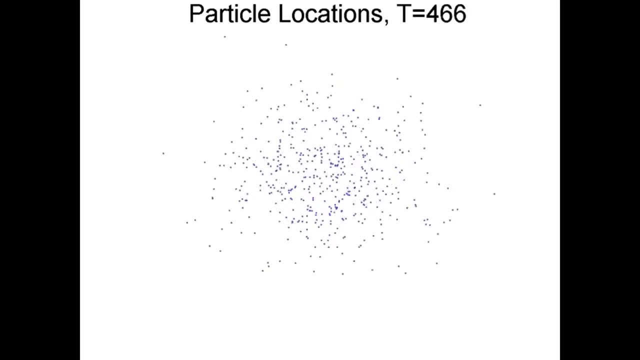 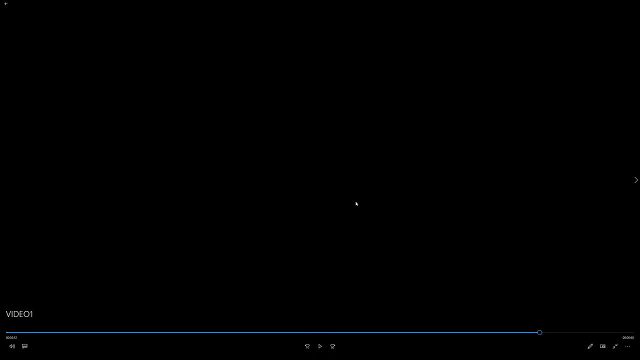 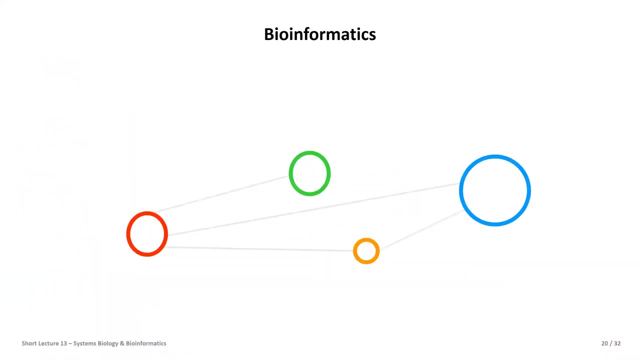 In fact, Monte Carlo simulations were named after the island of Monte Carlo because of the casinos using Monte Carlo simulations to understand their profits. I think that's enough for us to understand, And let's dive also, then, as part of the short lecture here. 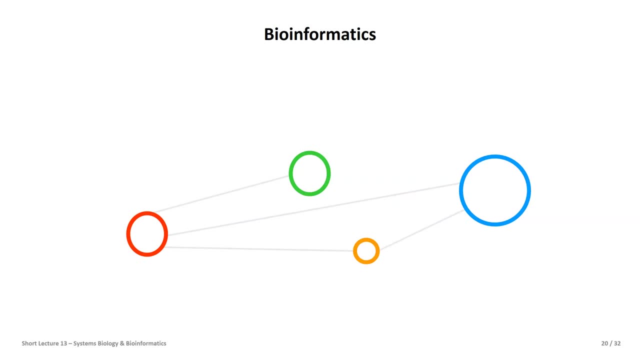 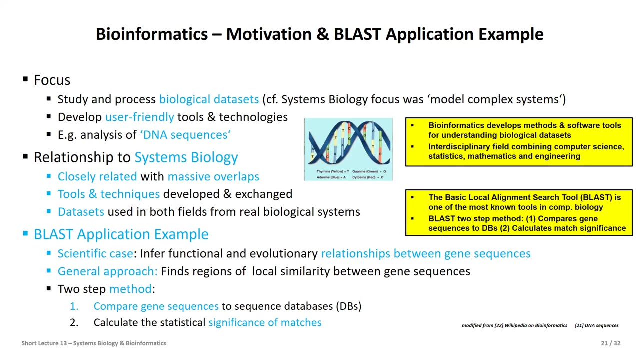 also in the second part briefly, this bioinformatics topic. So essentially with bioinformatics you have a very broad range essentially of really understanding, mostly studying and processing really biological data sets, And that's the point I want to make here a little bit. 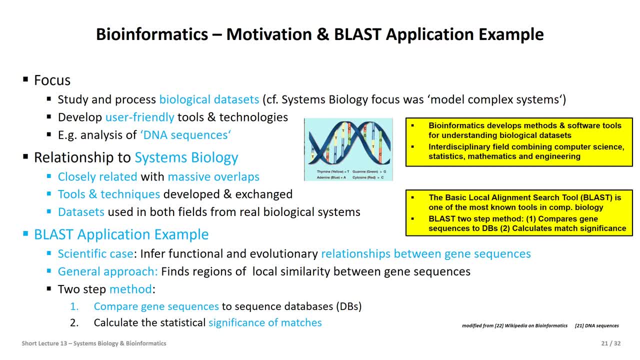 The role of data sets, the role of data at large in biology and bioinformatics, which is an important part of it, And I have here one example application which is known, called the BLAST application, so-called Basic Local Alignment Search Tool, which basically is a two-step method. 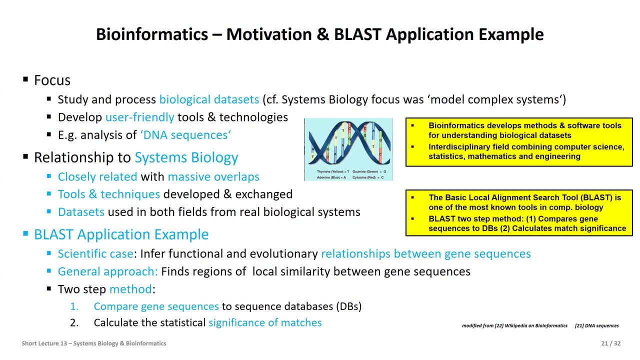 It first compares gene sequences to a certain database and then calculates basically the match significance of a new string that you basically give as input. So in this sense we go as this particular idea of an application But of course take away the message. there are many different applications. 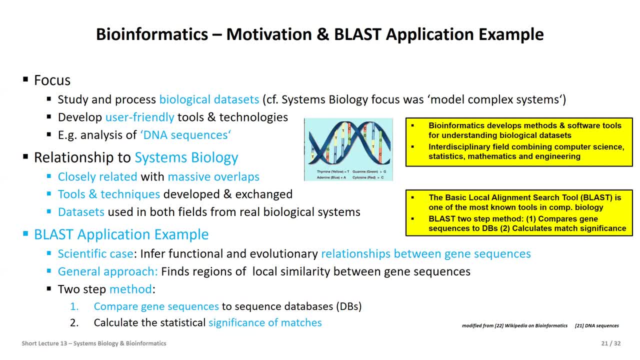 I think COVID-19, the research on data says it all to really understand what's happening there, what happened there, which you basically have probably seen from different approaches, from systems biology perspective, But they have, of course, massive overlaps with systems biology. 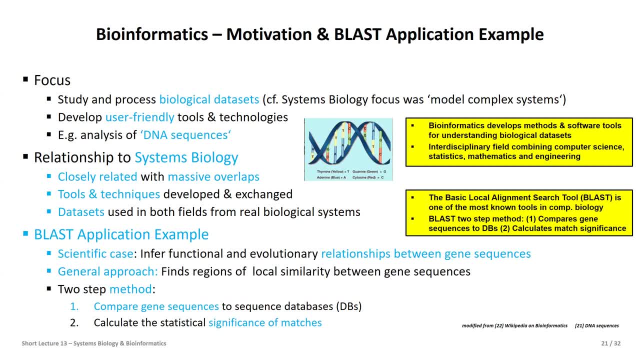 But on the other hand it's also used in much more areas where data play a role, several tools play a role and techniques which are rather called bioinformatics. So here the idea of the BLAST application is really find the functional and evolution relationship between specific gene sequences. 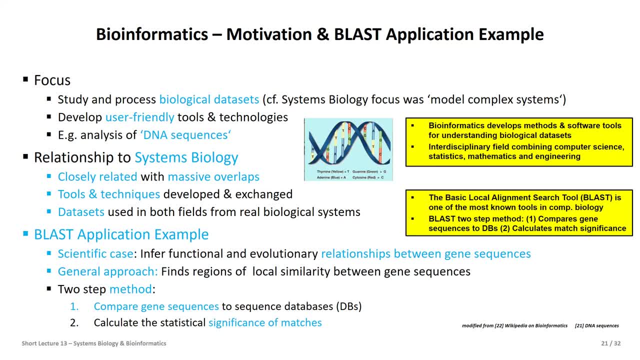 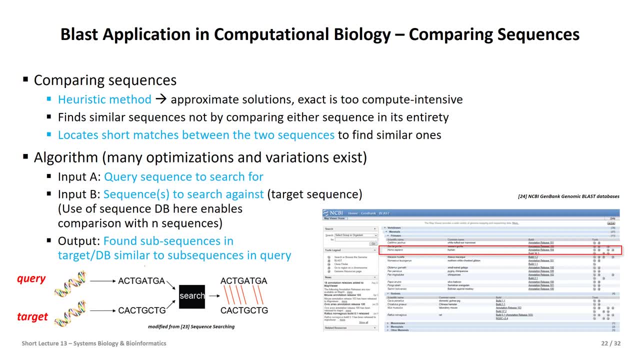 something we already had a little bit in the first part of the lecture, So we can go a little bit faster here. compare the sequences: you have a circle target that you have and you query basically the sequence to search for this against a specific target sequence and you find sub sequences in this. 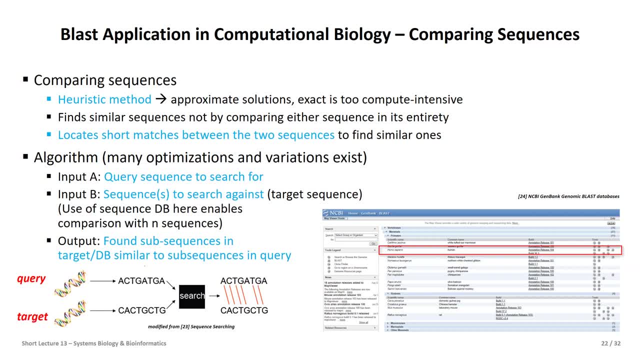 target database, which is similar to the sub sequences that you query for, which is essentially a little bit what you have here elaborated, and for this you can say that you use large databases, like you see here: the ncbi gene bank that has, for instance, also the human genome parts and also of 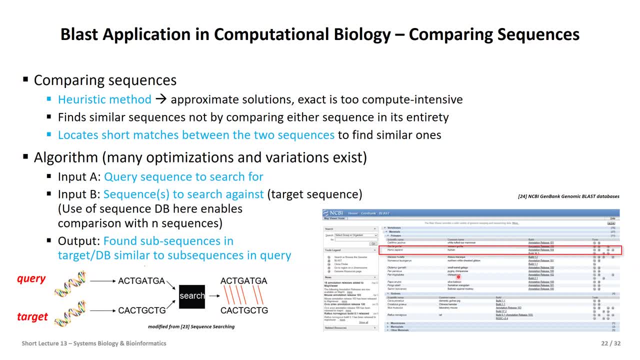 course many others. you see here elements, chimpanzees for instance, as well, and here you want to have the short matches between the two sequences, essentially, and once again i think, courses from park melstead in our, you know, universe of ice, and or, more generally speaking, bioinformatics courses. 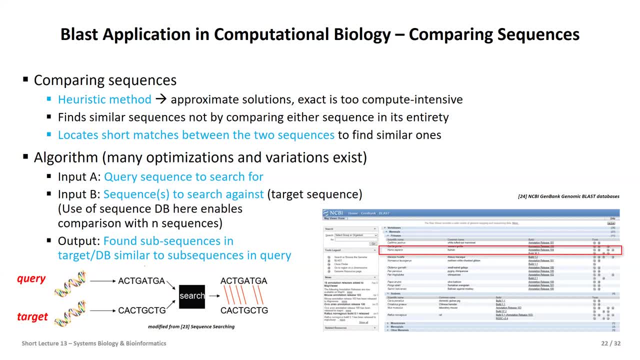 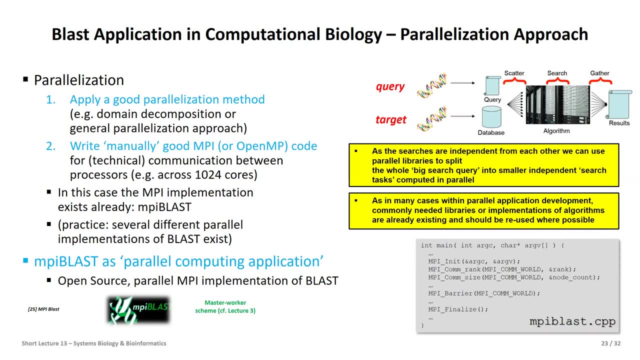 make sense to really understood that the better view and the bigger view on it not just bound to hpc, but we want to understand a little bit why we can paralyze it, why, basically, we can good apply a very good communication and parallelization strategy between different cores. here we have. 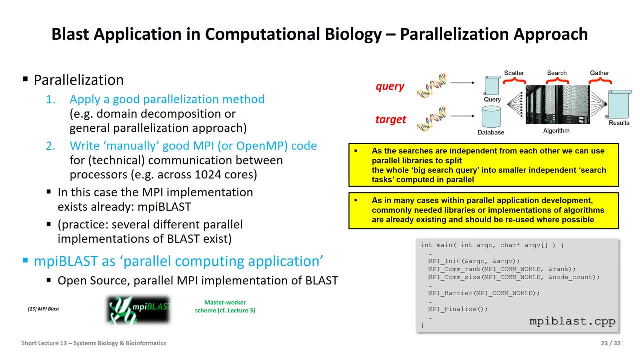 an mpi implementation of this blast application, which is open source and deploys a bit the master worker scheme, because you can imagine that you have different queries you search for and you have this database where you select the target. so you can imagine if you scatter this out and then 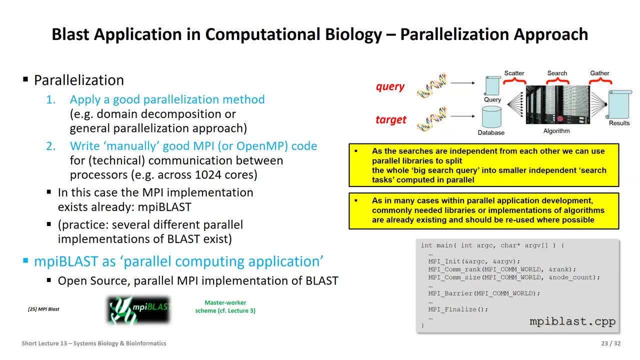 search in parallel, all these kind of matches that we discussed- you can then gather the result in parallel. so- and this is something where you know, basically these big search queries can be split in smaller, so to speak, independent search tasks, which then can beautifully use hpc, and in the end you want to. 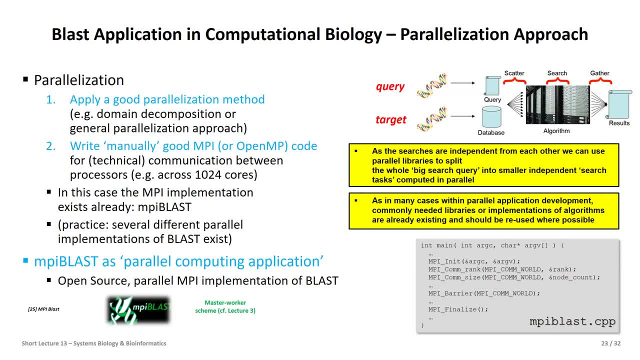 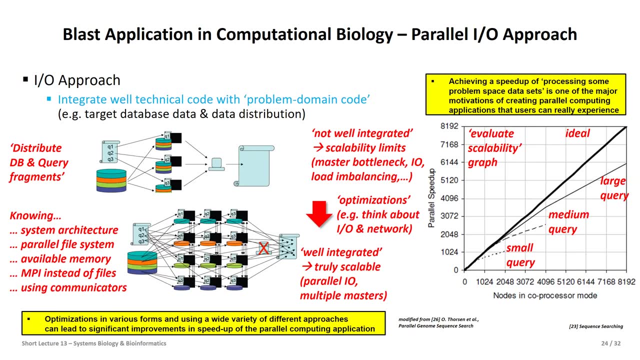 let's say, use mpi then to gather the results again, and that's actually done in this code so you can use it. it's production ready- and of course also in many of these parallelization codes in bio informatics. here the io approach just shortly, because we're also thinking about what we 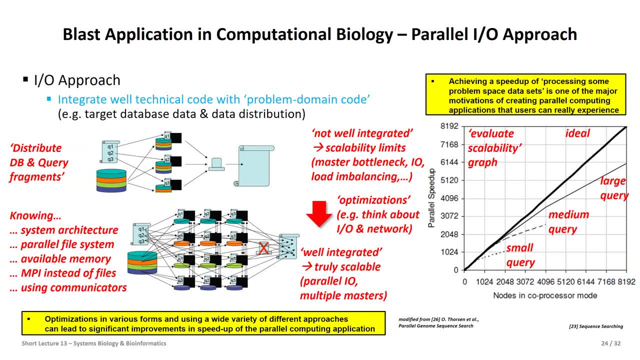 learned in terms of our parallel io, also of our thinking about io, really matters when i want to do distributed computing and parallel computing. you see here how that a little bit works is if you have this distributed database and query fragments only and they work all on the diff. 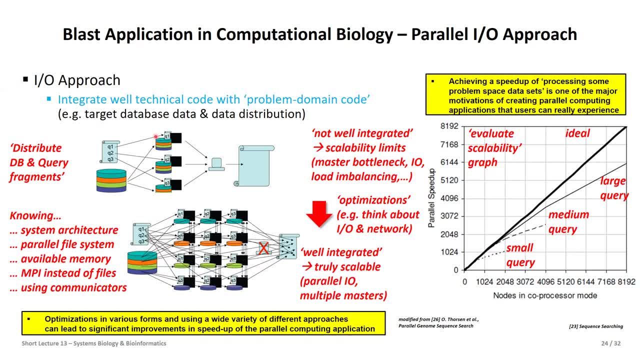 let's say, on the whole database. this could mean you know basically also um a little bit you know of a more or less performance. so what you want to do is that you really understood your problem very well with the data distribution and so on, so that you know the system architecture that you can. 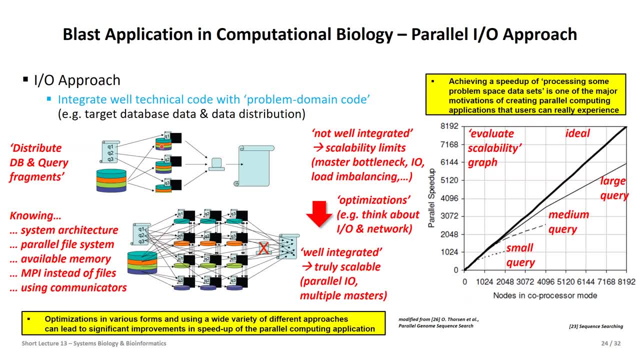 of course also split the database here right, let's say concurrent access to this databases that we have anyway, as we learned in parallelio, and for this we basically don't gather the result only, let's say in one computer part, as a master worker in a way suggests. but here we could with. 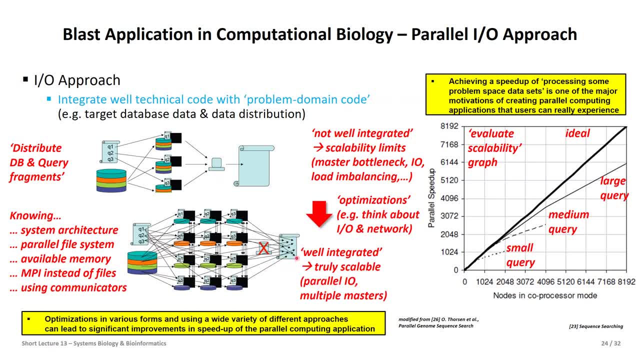 parallelio, i can directly write results in a different parallel child shared file. and with this you see that, depending on the number of queries, really, of course, you can really scale quite nicely, not directly linear, but almost, let's say, you know, in a way, towards linear performance. 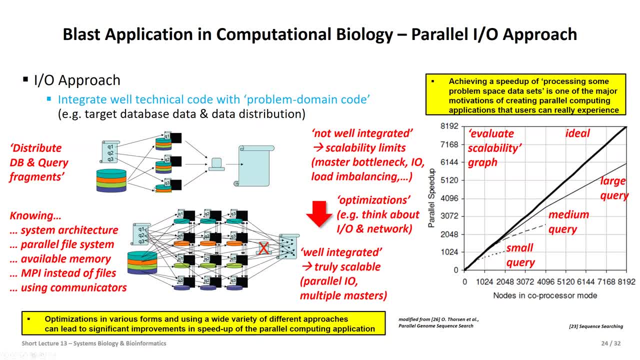 and just by knowing exactly how you can different do here, parallelization strategy of this very trivial, simple problem of search, which of course i know that the data distribution is very important to understand and to work with the data distribution. but i would also like to add to that is there is. a very good answer in the data distribution that the data distribution is very good and very difficult to understand because it's very difficult to understand. but it's very difficult to understand because it's very difficult to. of course, given the amount of data, it's not at all trivial. 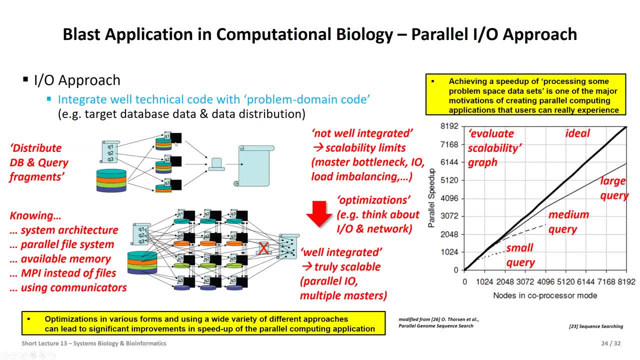 But of course trivial from the perspective that you just try to find some subparts of strings- And this could be, of course, nicely parallelized- And then you see how much speedup you can gain here in terms of adding more and more. 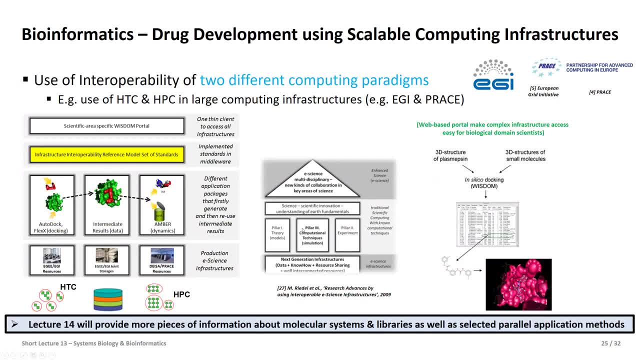 coprocessors here to the game. These are just examples. obviously, When you do this to a higher level, you see here drug development, using scalable computing infrastructures, where we used high throughput computing for instance in the past to do tools like autodoc and doc. 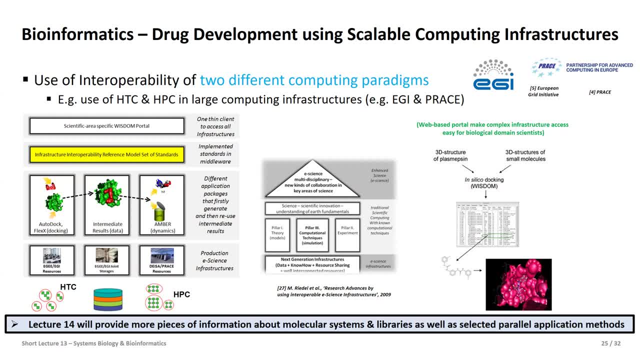 and see if there's a potential drug coming out. if it docks at all to the different legions, Then you have a sort of intermediate result that, of course, is docked, So in a way it could be a potential drug. 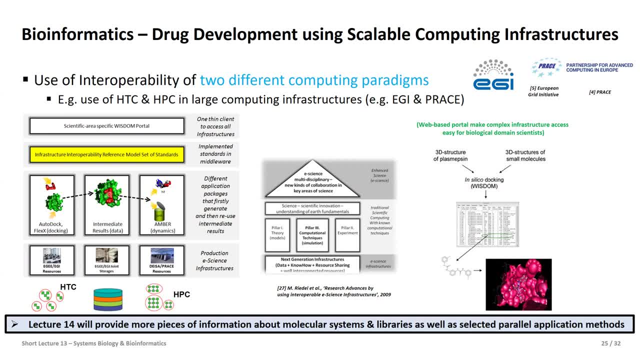 but not really, because we have force fields. That means we have to evaluate yet something we called molecular dynamics, and with amber and so on, with different packages, If this really will be, you know, stay together over time. So, and this is an important simulation of amber, 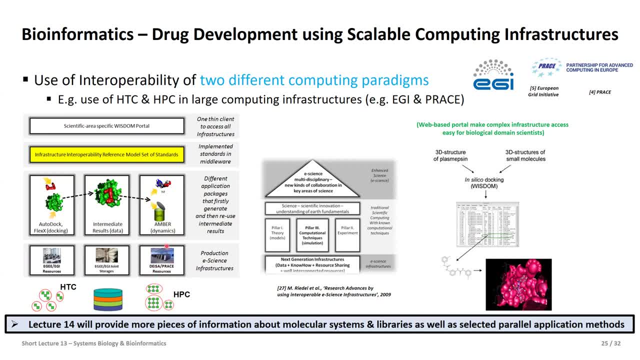 which is very computationally demanding and then really requires praise or HPC resources. So some of the bioinformatics problems can be done in the very HTC oriented fashion, but some of them really require HPC. What we did here basically then in silico docking. 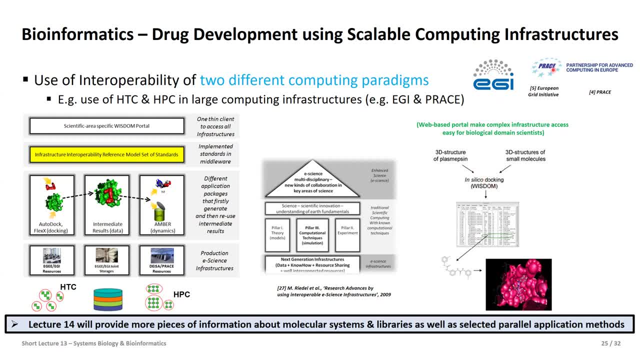 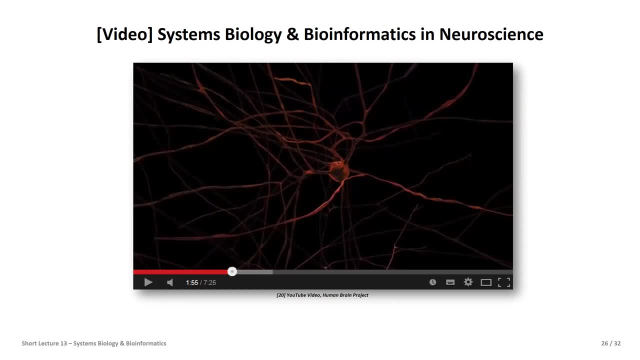 this is two-step approach And this used really high cutting edge HPC and HTC infrastructures, And we will talk more about molecular systems and library, essentially then also in lecture 14.. But basically this should be just a very brief intro in bioinformatics, how you think about data. 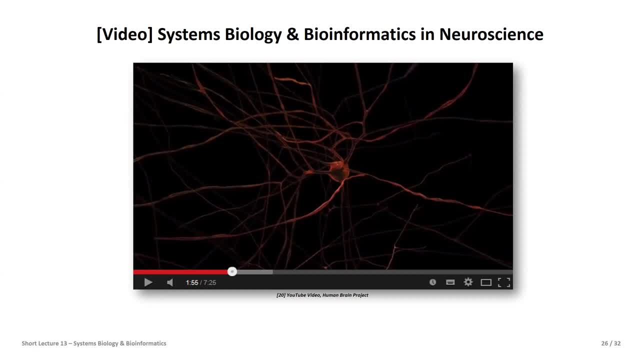 And let us now think about how we can go to the next steps in systems biology and bioinformatics, by revealing a little bit the human brain project, where we are also involved in in Jülich, at the German site, very intensively, And it's a very interesting project. 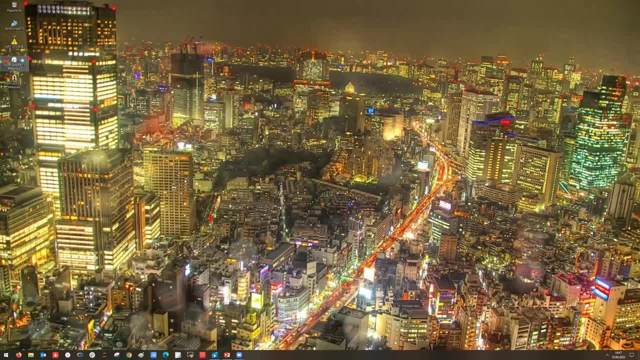 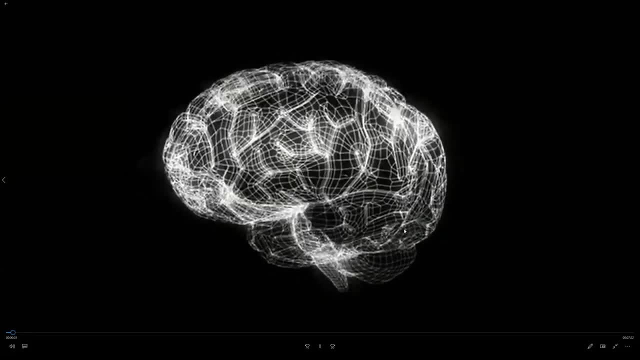 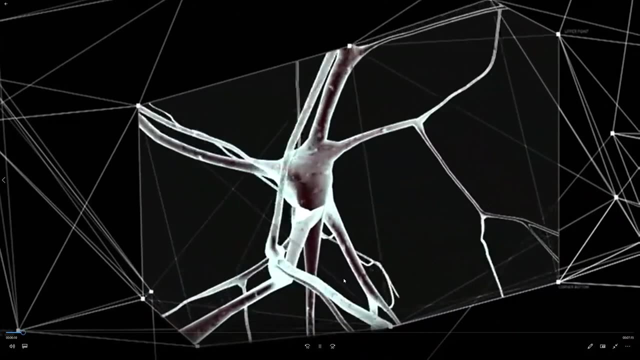 a very, let's say, demanding project, really, and that's what this video should entail for you. A hundred billion neurons connected by a hundred thousand billion synapses: The human brain is the most complex machine we know of and the most mysterious one. 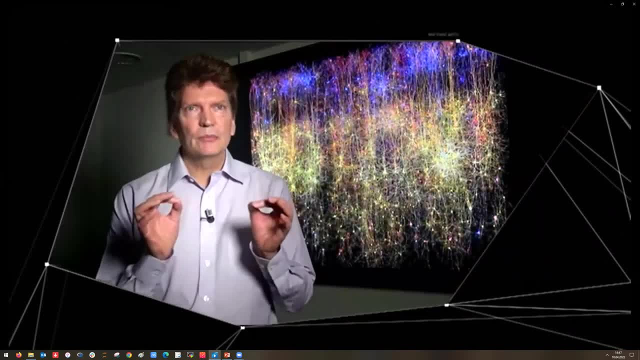 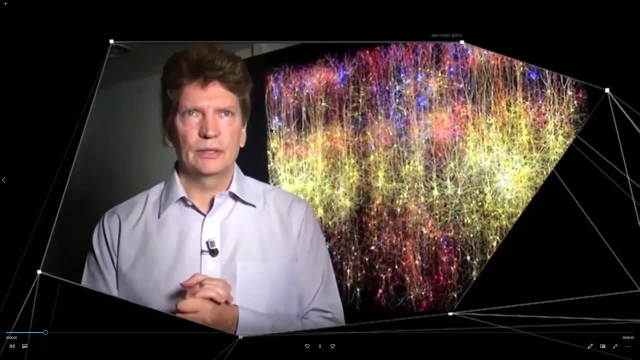 We face huge issues in neuroscience to understand how the pieces of the brain fit and work together. We face huge issues in medicine to understand how to objectively diagnose, to understand how to objectively diagnose and treat brain diseases. This is a big, big challenge. 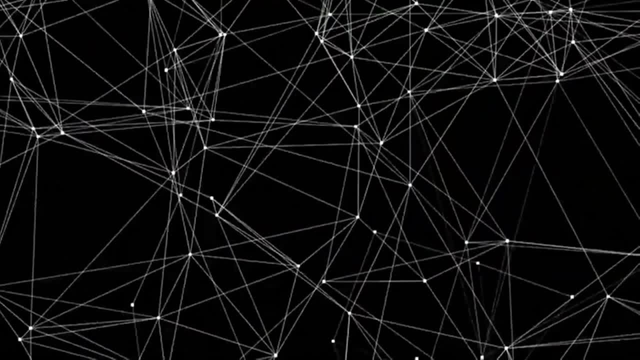 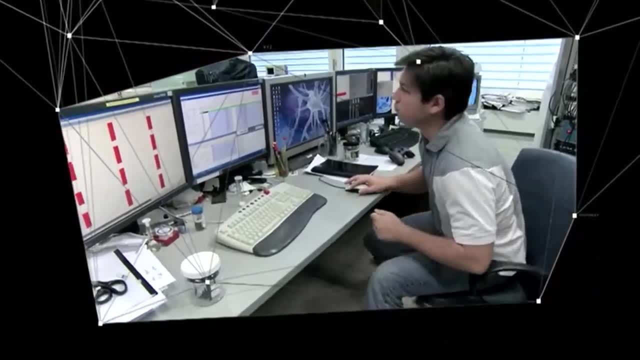 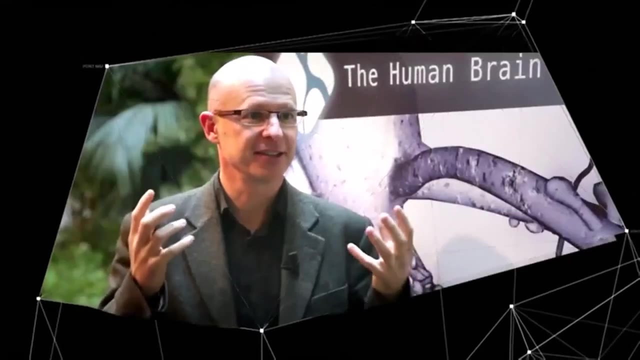 It'll have an enormous impact on the health of the aged. European researchers propose a radically new approach to study the human mind. Their idea is simple: to simulate a complete human brain in a supercomputer. We have a giant intellectual problem to solve here. 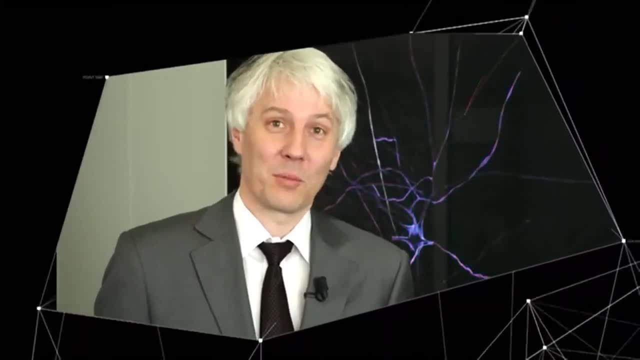 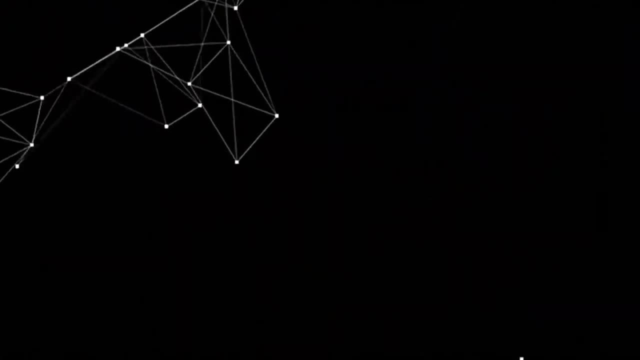 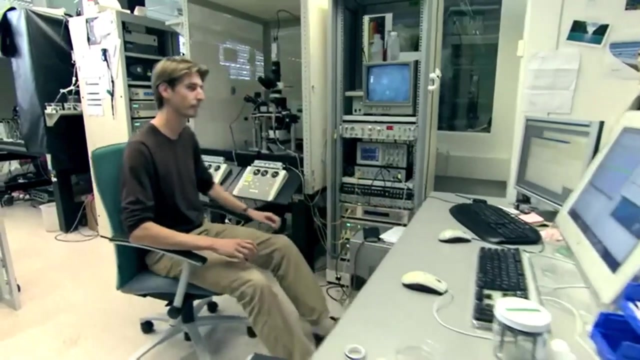 As a scientist, I mean. it's really the central project for brain science. It could revolutionize computing the way we do it today. The Human Brain Project brings together hundreds of scientists from leading European research institutions. It is one of the most ambitious neuroscience projects. 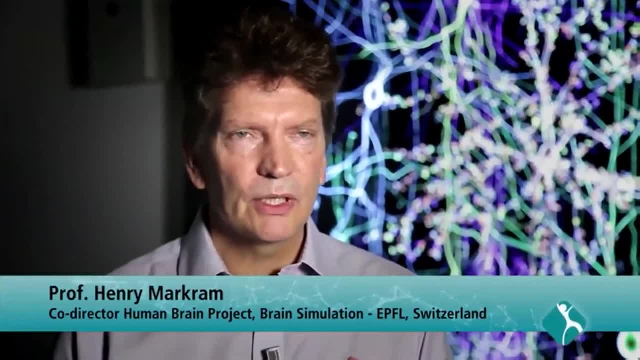 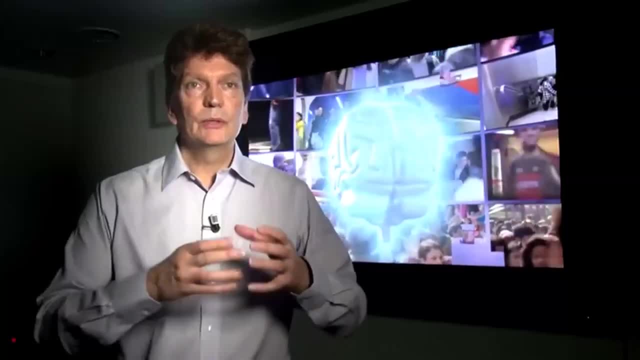 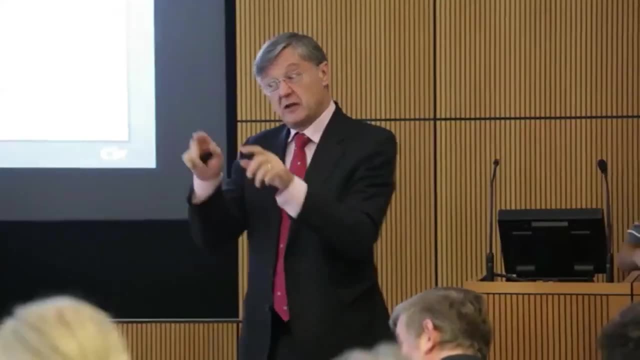 in the world. What we are proposing is to establish a radically new foundation to explore and understand the brain, its diseases, and to use that knowledge to build new computing technologies. The project is coordinated by EPFL, located in Lausanne, Switzerland. 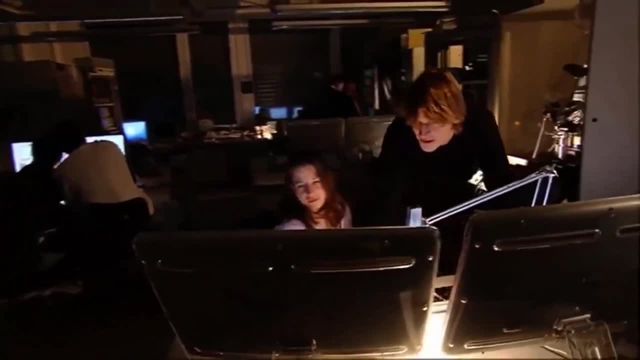 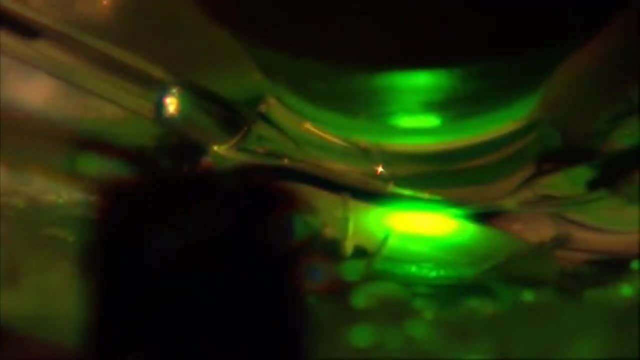 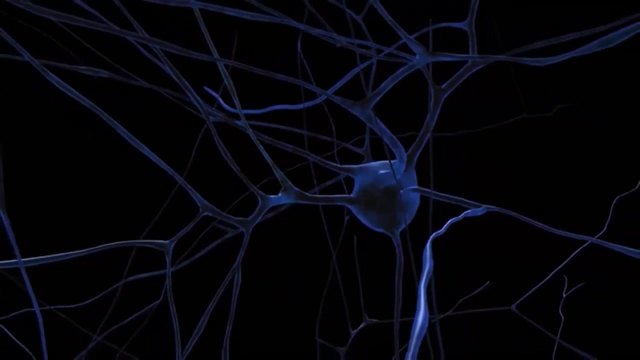 The researchers will systematically study neurons, the building blocks of the brain. They will collect and consolidate all the biological data produced by scientists around the world. They will integrate this knowledge into a massive simulation running on a supercomputer. The result will be the most accurate model. 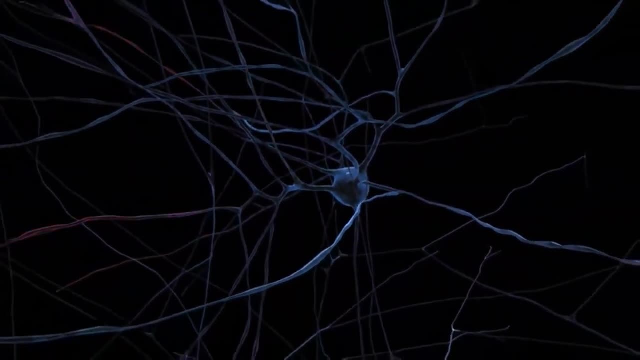 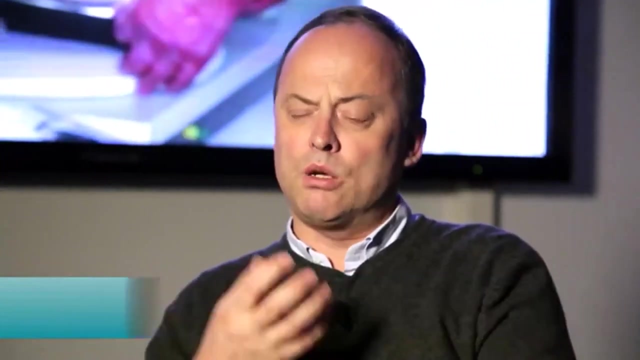 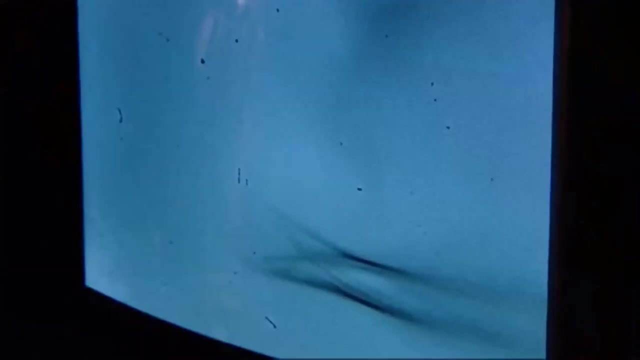 of the human brain ever produced. I'm really thrilled to be part of this and to help neuroscience to have a more coordinated effort To understand the brain and to exploit the brain, To really use what's in the brain in computational principles and to derive new technologies. 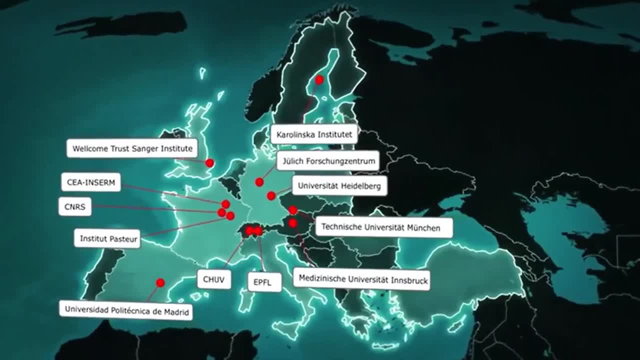 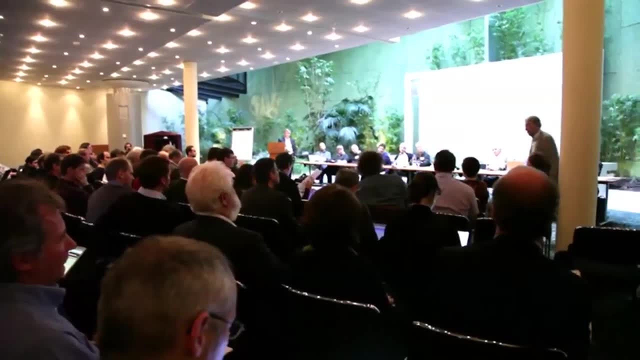 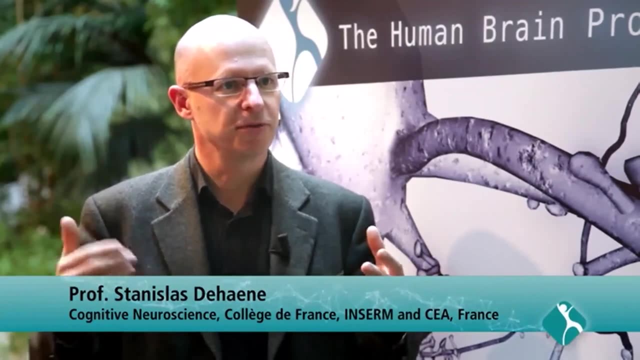 From an original group of 13 institutions, the HBP now encompasses more than 80 partners across Europe. The human cortex is organized into specialized regions. We need to understand what these different regions are doing. Some are specializing for language, some are specializing for vision. 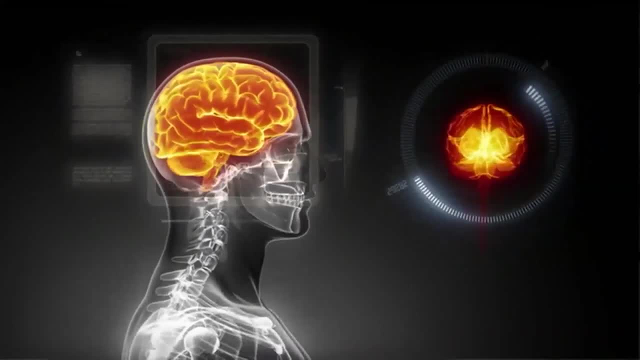 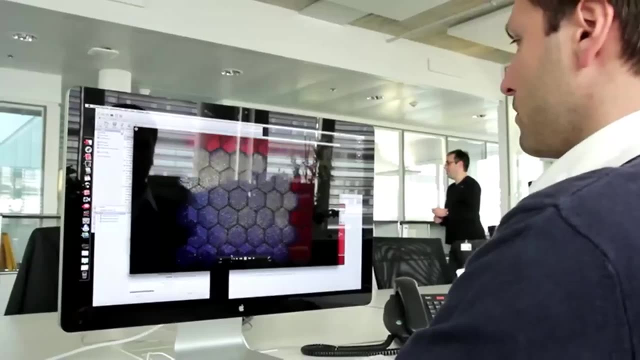 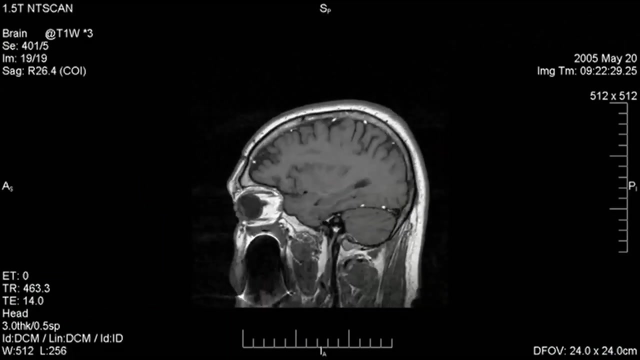 So we will create systematic maps of the human brain, trying to understand each of these subsystems And trying to understand what are the specific parameters, so that they can ultimately be brought to simulation. Brain diseases have become more common. They become an immense burden in the Western world. 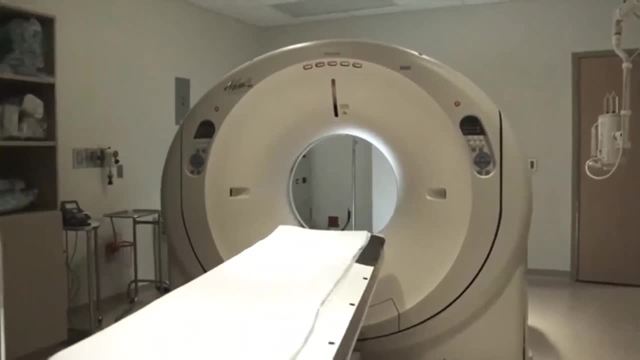 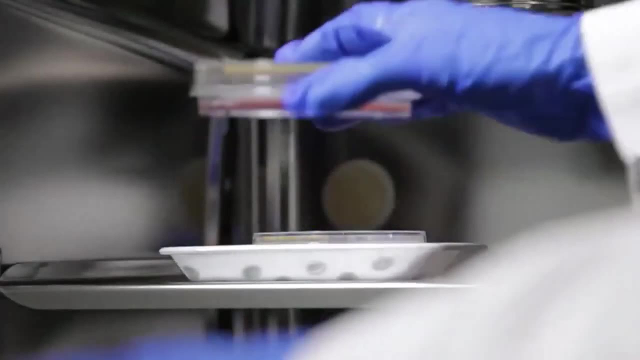 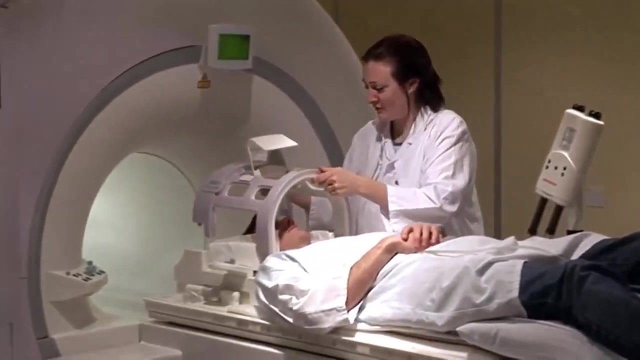 In Europe, they cost more than heart diseases, cancer and diabetes all put together. Scientists will work closely with hospitals to find new treatment to neurological disorders. They will collect medical data, such as brain scans, in order to develop better ways to diagnose diseases. 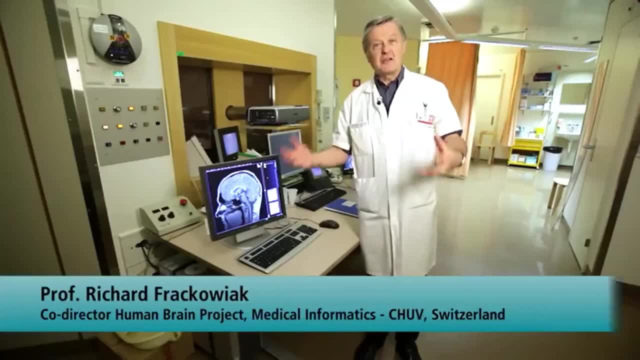 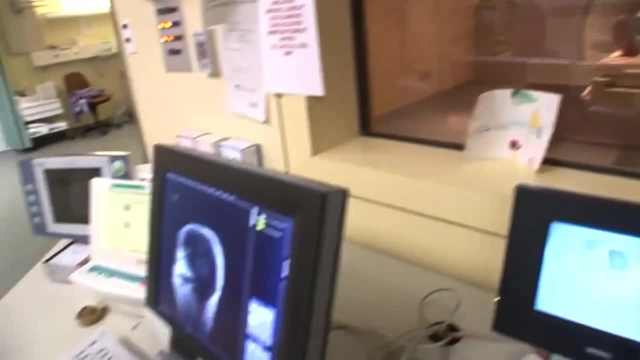 It involves trying to make sense of the enormous amounts of data we collect on all our patients And using those data In order to define the brain, To define their diseases better, And to do that we need first to be able to bring the data together. 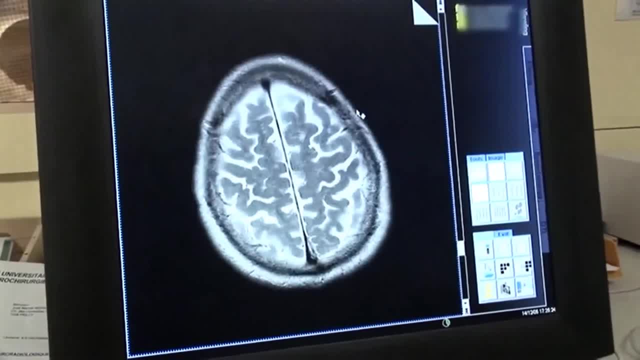 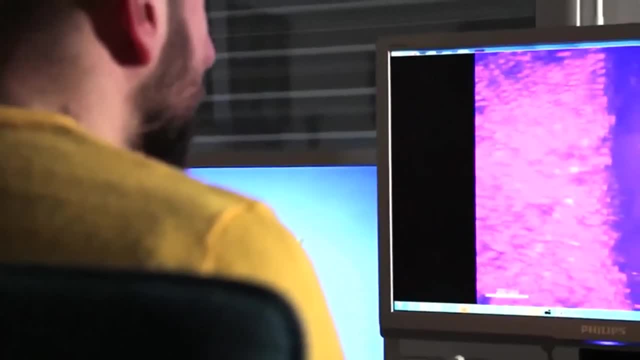 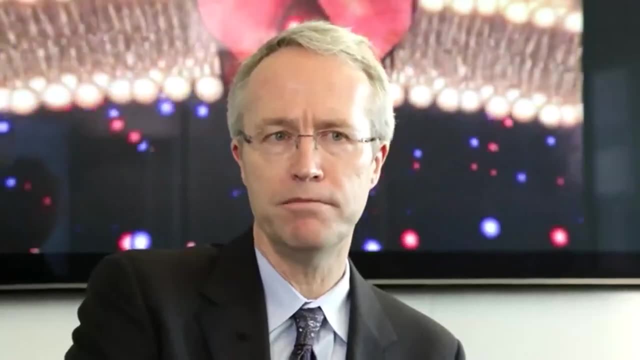 So we need data basing, And for that we're going to need really high powered computers to be able to what we call data mine. We now have a blueprint to understand the molecular architecture that defines the development and organization of the human brain. 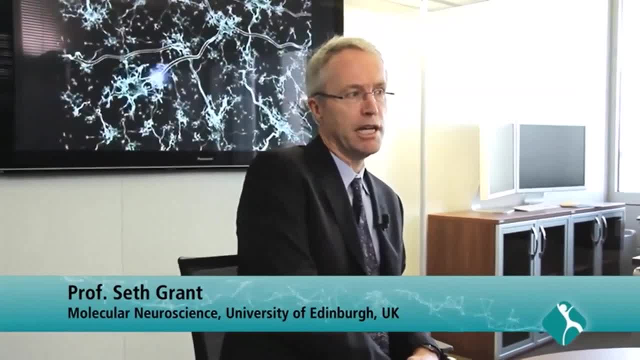 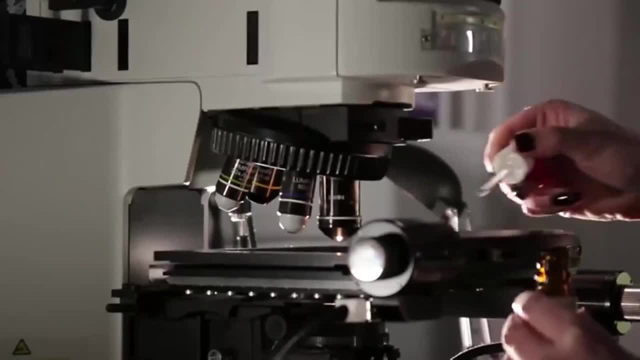 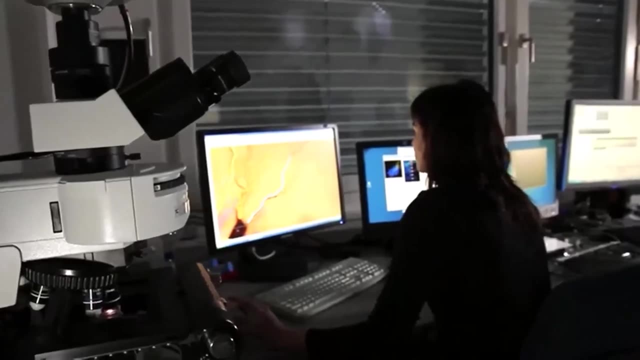 But it also gives us the fantastic opportunity to understand how the DNA mutations that cause hundreds of different brain diseases produce those diseases. There'll be ways of testing potential drugs where you won't need to use animals, Where you'll be able to use something that approaches the human. 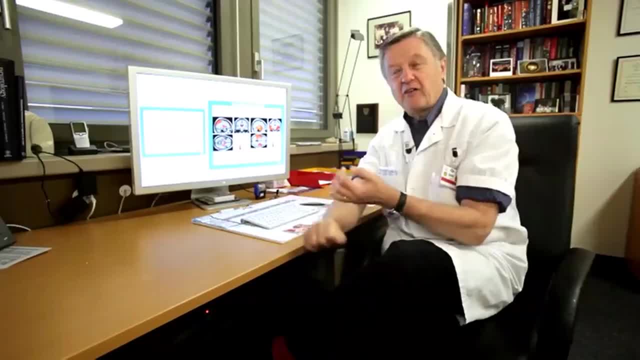 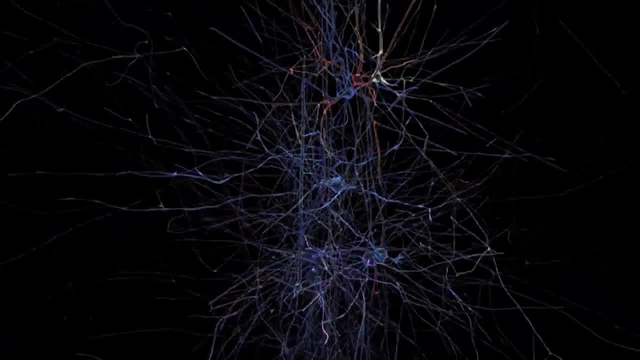 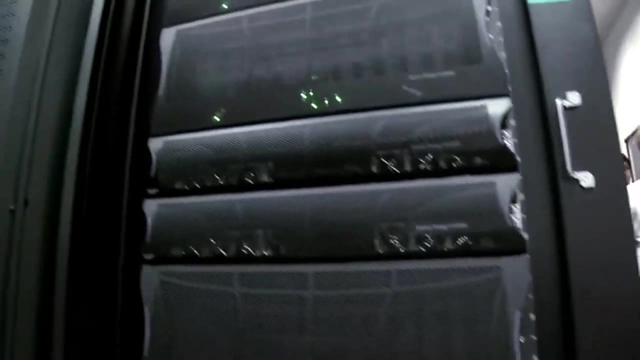 And where you'll have some information of how good the treatment's going to be. to correct the defect, The simulation of a complete human brain will require supercomputers that are a thousand times more powerful than today. The power of today's computers is by far not sufficient to compute this complex system. 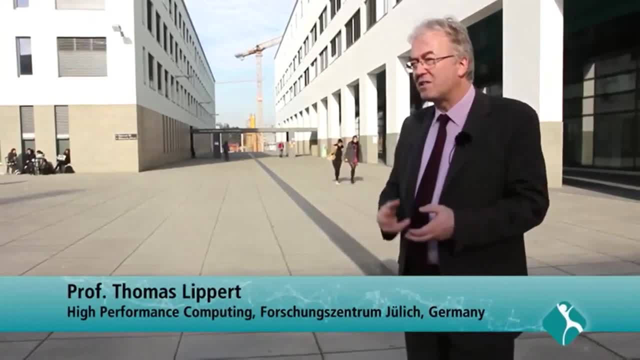 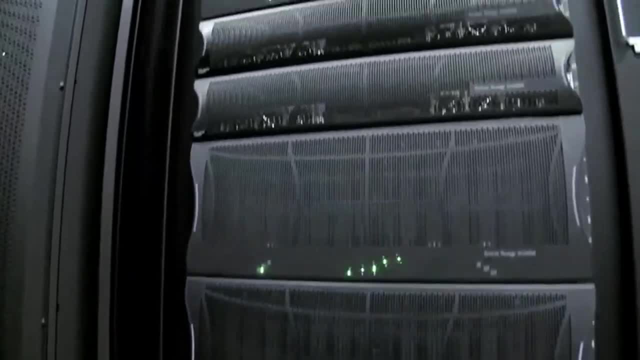 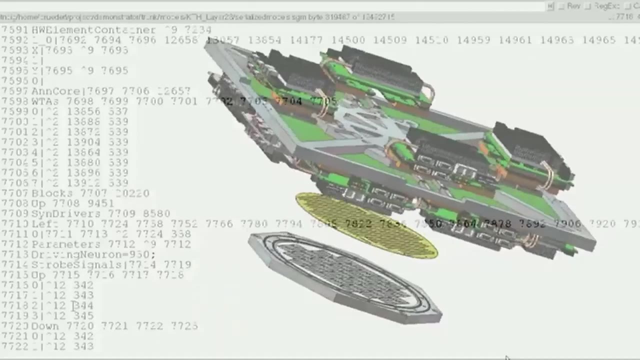 Of course, we have to pool resources in order to satisfy the huge demands. The project will stimulate the development of new supercomputers. By understanding how cognition works, it will help to design radically new devices called neuromorphic computers. They will combine the power of the brain. 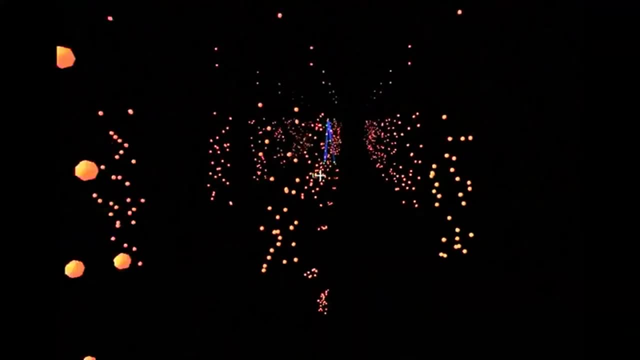 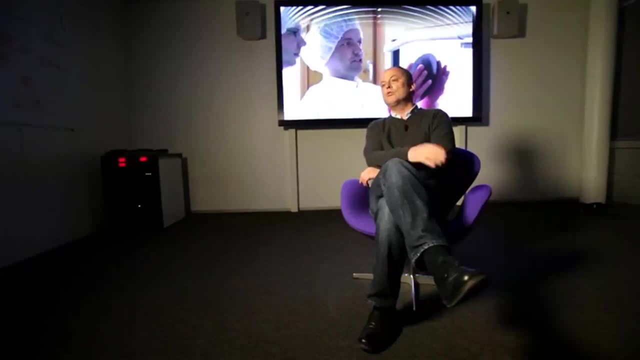 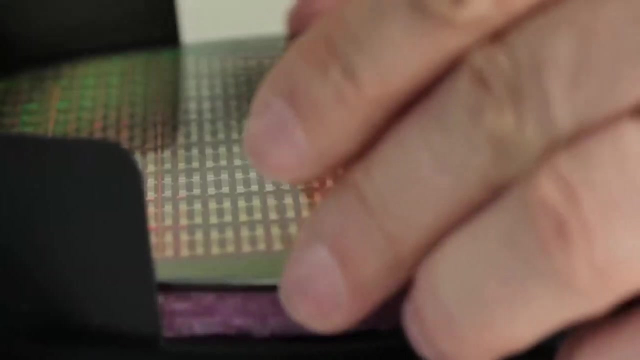 They will combine the power of microelectronics with the flexibility of human intelligence. If you want to solve a new problem, you need new software. You don't do that. in your brain, You learn, and you are able to learn to handle completely different situations. 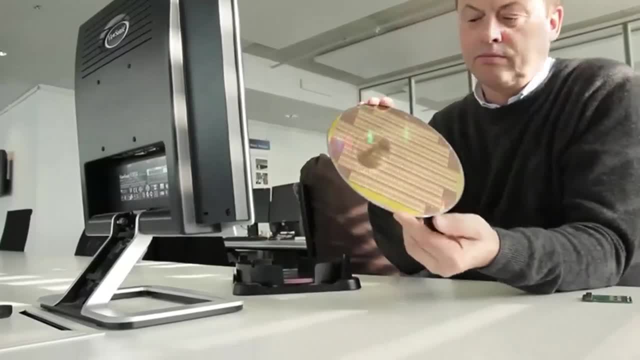 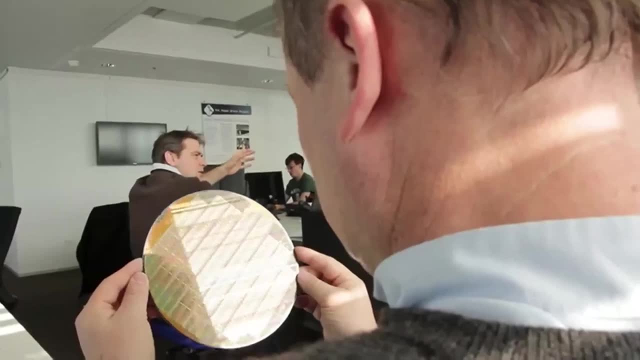 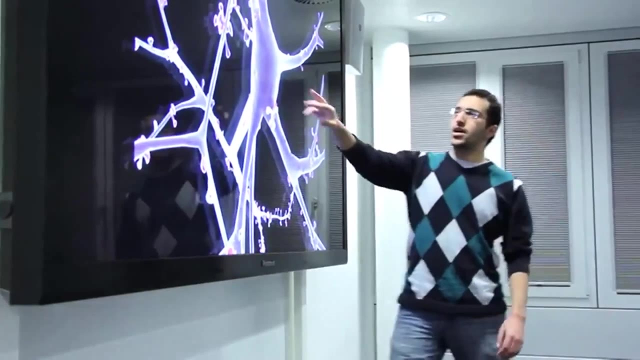 even things which you have never seen before. These are systems that are directly modeled after the brain, So what we build is physical models of brain circuits on silicon substrates. The Human Brain Project will create a realistic simulation of the brain. This new tool will be used to understand how the mind works. 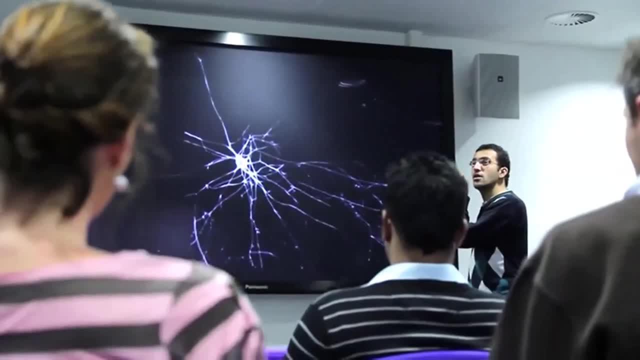 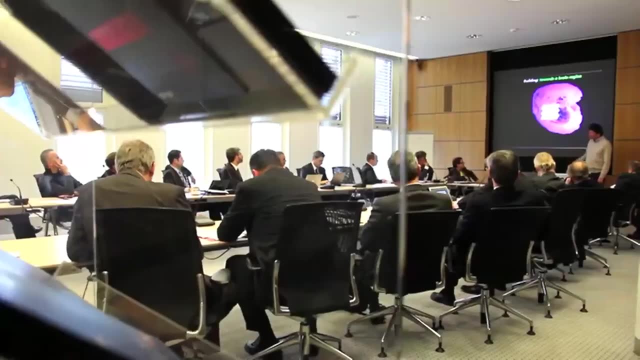 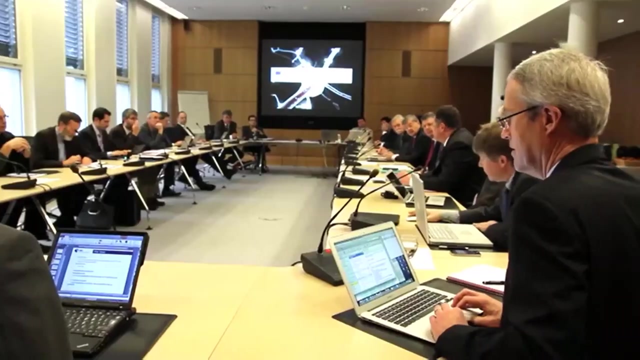 to study brain diseases and invent new electronics. To achieve this goal, more than 80 European institutions have already joined the project. The competence is distributed all over Europe in supercomputing and in neuroscience. By bringing so many different people together, 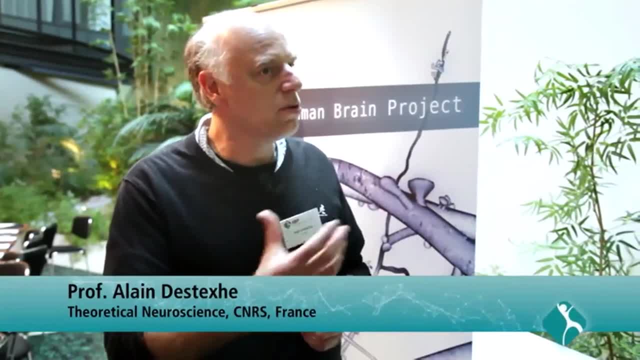 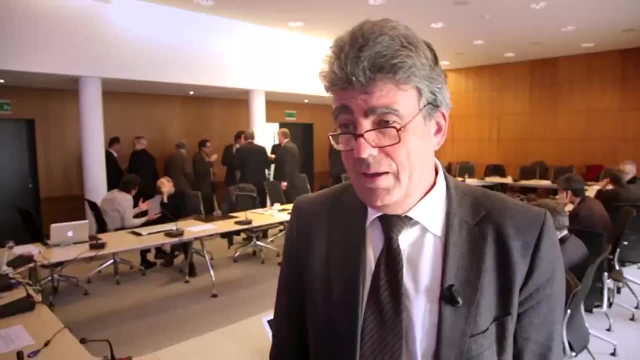 and making such a big community such a big project, we can do things we could never do with any other smaller scale project For Europe. this is kind of a big science project. I believe the 21st century will be the century of the brain. 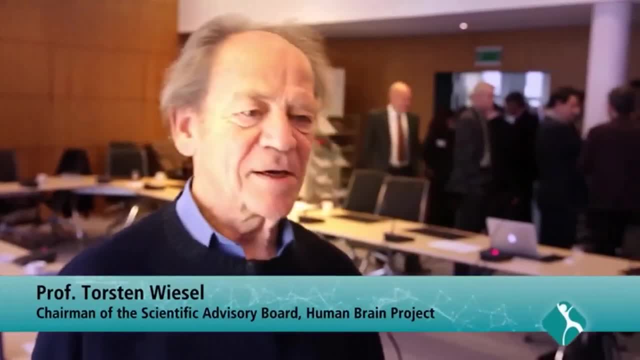 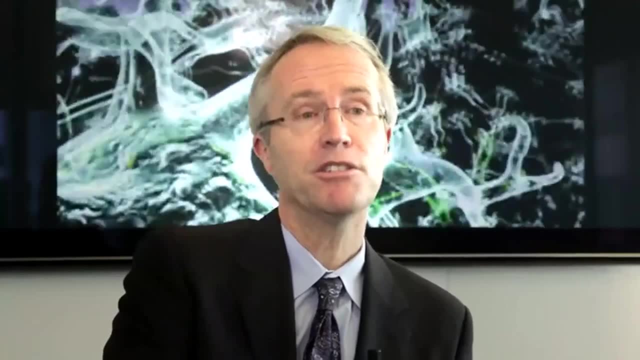 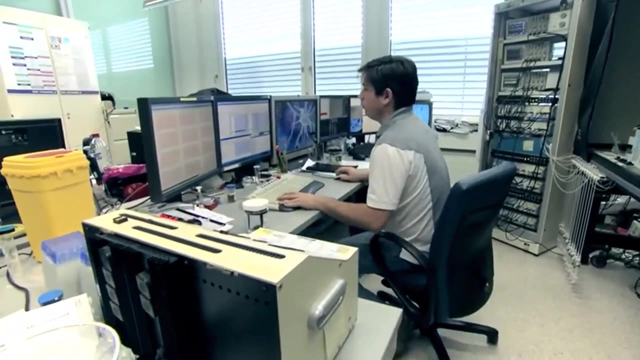 I think the project is a visionary project And it seems to me that the field needs this kind of initiative really to move forward, And I see fantastic opportunities in the future. The technology is at reach and the necessary knowledge available. It's like building a giant telescope to peer into deep space. 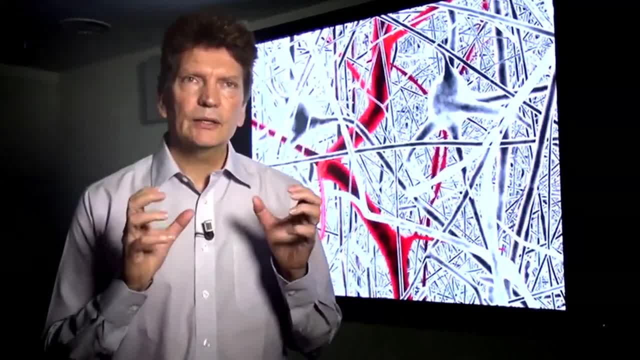 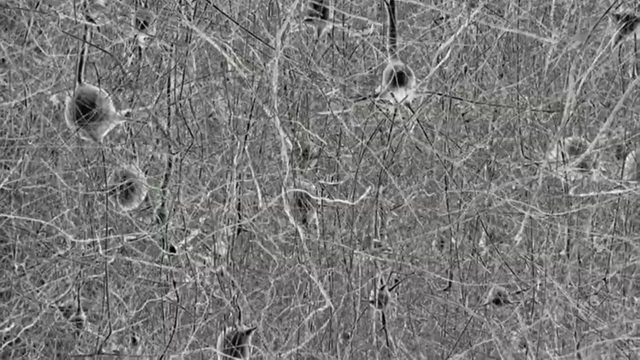 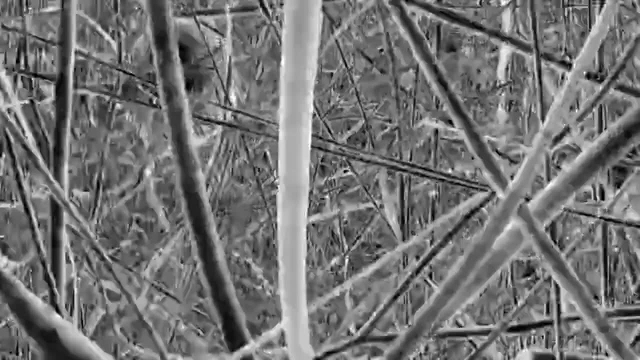 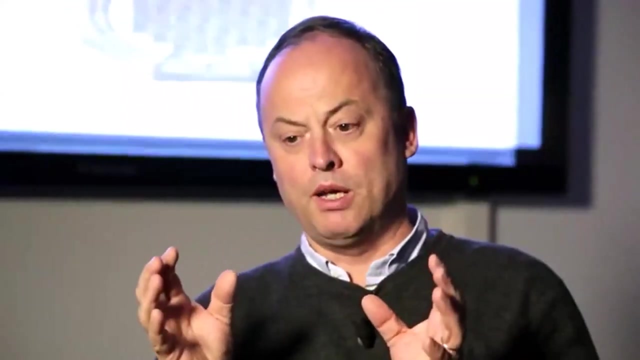 only that we'd be able to look deep into the brain and ask questions that are impossible experimentally and theoretically. It's an infrastructure to be able to build and simulate the human brain, objectively classify brain diseases and build radically new computing devices. We have what's called, in technology, a roadmap. 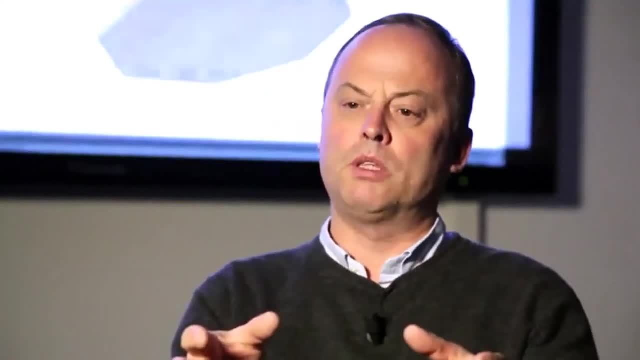 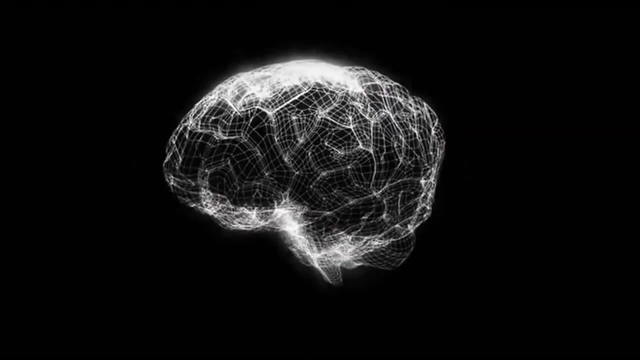 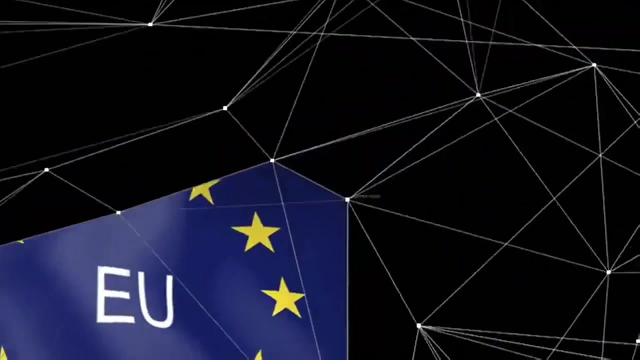 We know which technology will be used at which point in time in the project and the way we will scale up our systems so that they reach the complexity of the human brain. The Human Brain Project will put Europe at the forefront of neuroscience. It will deliver new strategies to fight brain diseases. 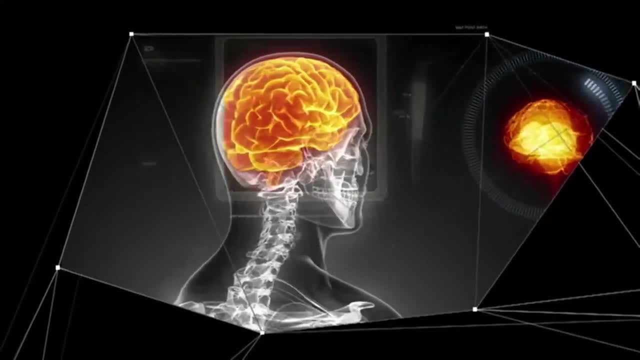 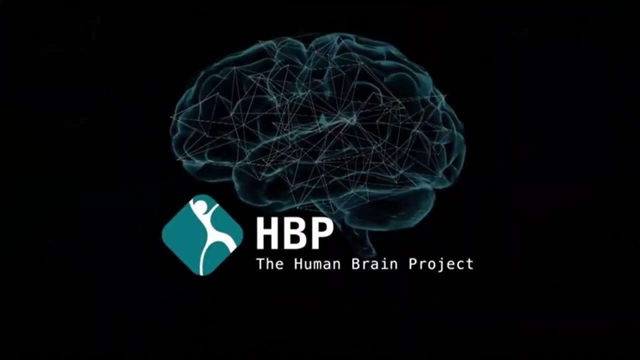 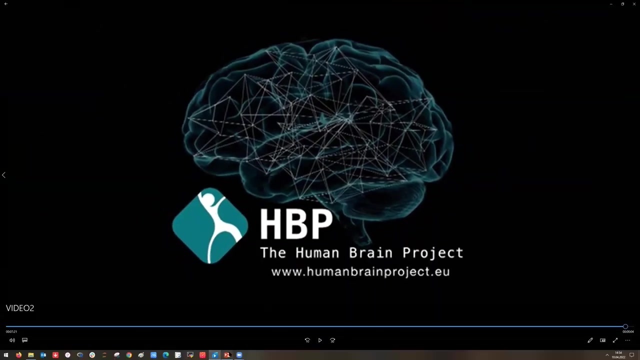 and it will revolutionize electronics. But first of all, it will offer a revolutionary new tool to study the most mysterious phenomenon of the universe: the human brain. So I think that's all Really. I wanted to leave you on the table today. 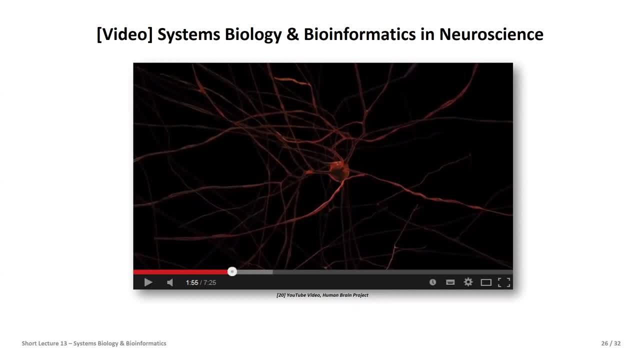 Of course, you hopefully take away the message that not only we can of course, understand and perhaps tackle diseases Also here the idea is thinking about that the brain is very energy efficient- right When it comes to watts, in a sense- and being very flexible. 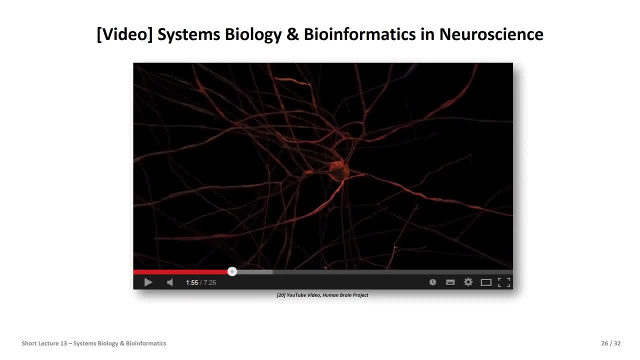 So how we can derive this knowledge to build new supercomputers which are maybe modeled after the human brain, which basically is a field, then, what we saw a little bit in the neuromorphic computing context. So in this sense we are done for this particular part of the short lecture. 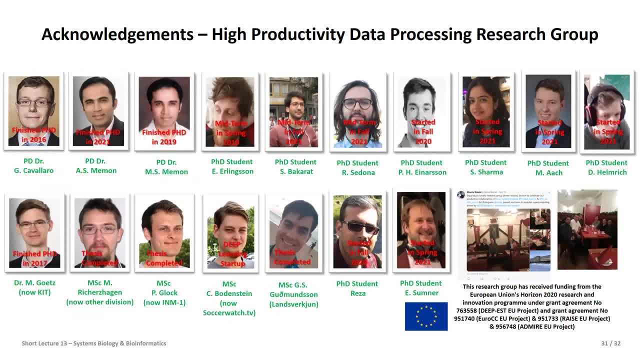 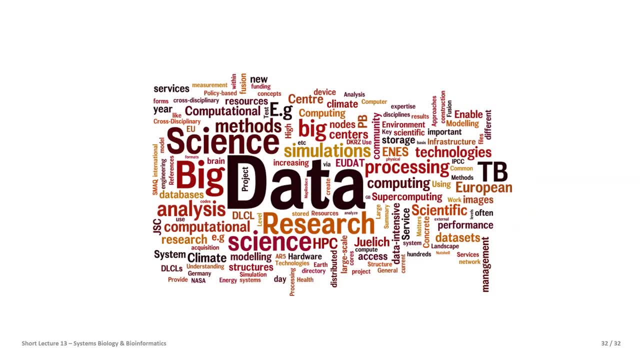 some references and we will pick up some of the elements we discussed here in the short lecture 13.. Again in the short lecture 14 as well, basically, where we discussed then again of molecules, systems and material sciences. So see you then.